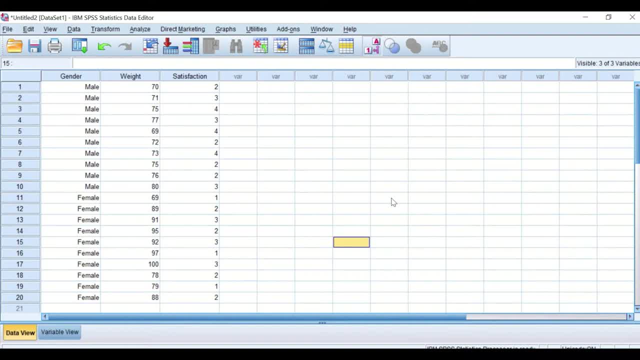 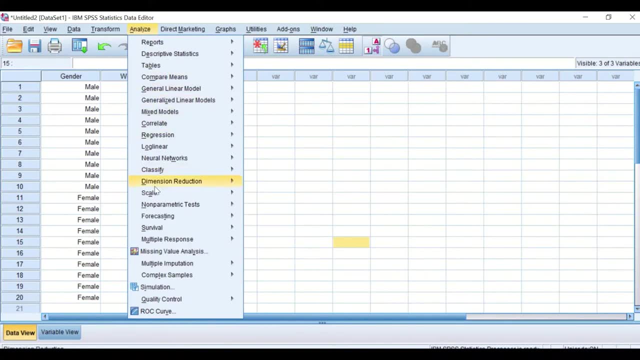 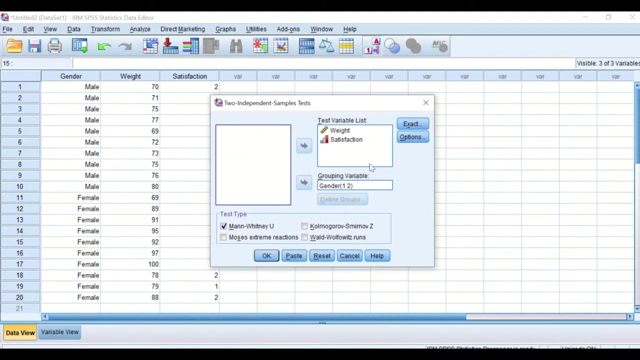 So to do the Mann-Whitney U test is very straightforward and easy test: Click on the analysis, scroll down to non-parametric and then scroll down again to legacy dialogues and scroll again to two independent samples. And I have to reset this and a window will appear and we need to sort and transport these variables and cases into relevant suitable boxes. 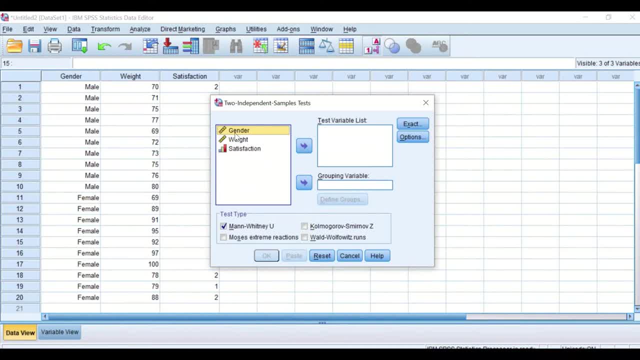 So we need to test this variable. We need to test the weight to see if there is a difference between the male and the female in terms of the weight, And also there is a difference between satisfaction in terms of the agree or don't they agree with specific criteria. 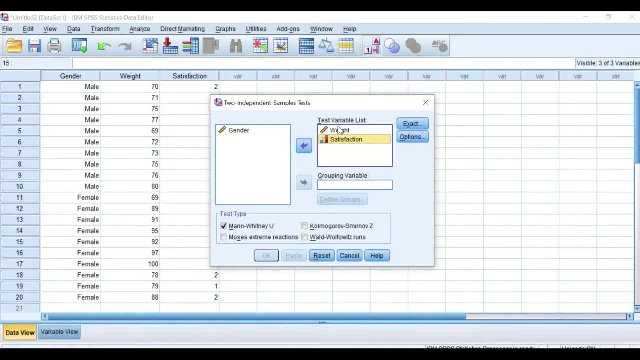 So satisfaction is also in a variable list. Now we want to group the group. It's based on the gender- male and female- And we need to click on define. group one: We give it number one. group two: We give it number two. 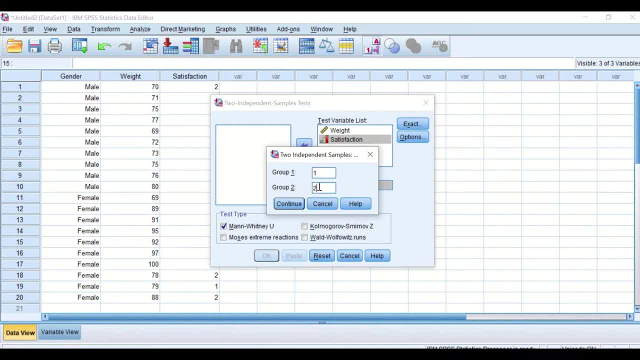 Why did I select one and two? Because I labeled one of these ones. I've labeled these as one and I labeled these as two. Click on continue And then I will select here the man with the new test, And then I will click also on exact and I will stick to asymptomatic only. 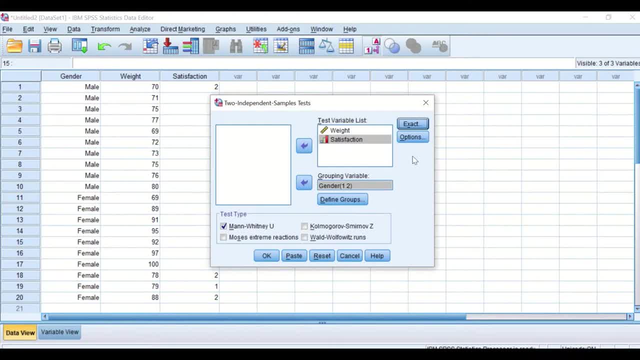 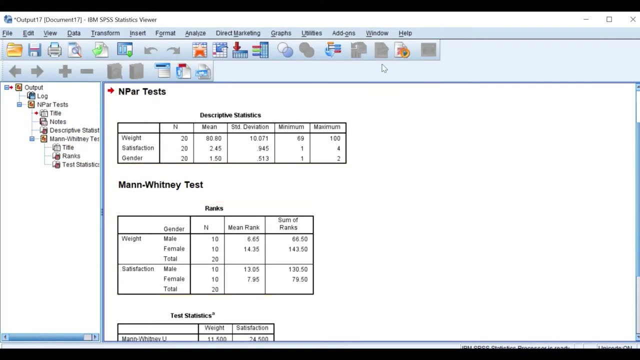 Click on OK, Then the options is not that much. unless we need to get some descriptive, We'll click on descriptive, Click on continue, then click on OK. SPSS output will appear in there. as we have seen Here, we have 20 cases, 10 males and 10 females. 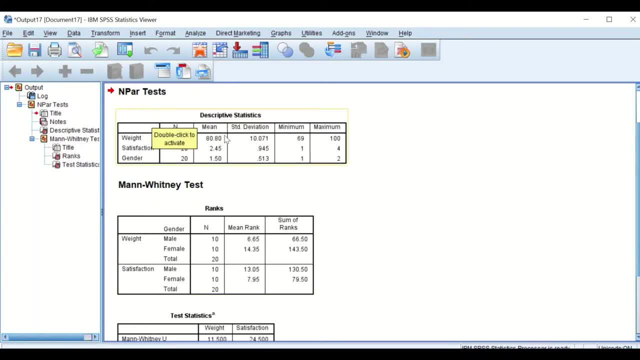 And the mean for the weight is 8.8 for the whole group And for the satisfaction is 2.4.. Now if we look at the rank, this is what the software has done. Rank them: there are 10 male, 10 female. 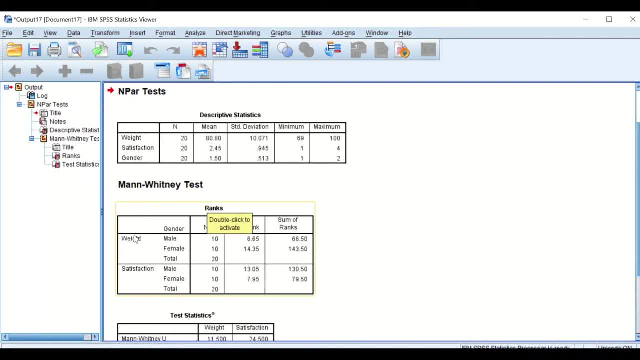 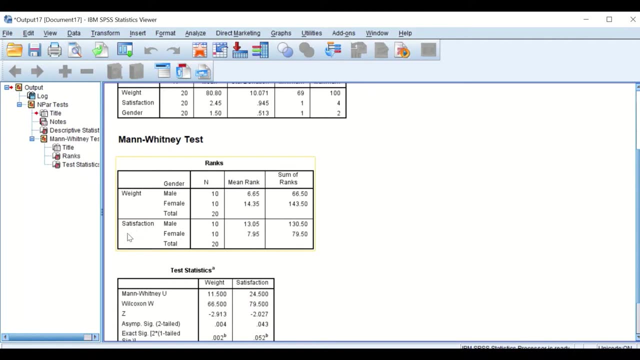 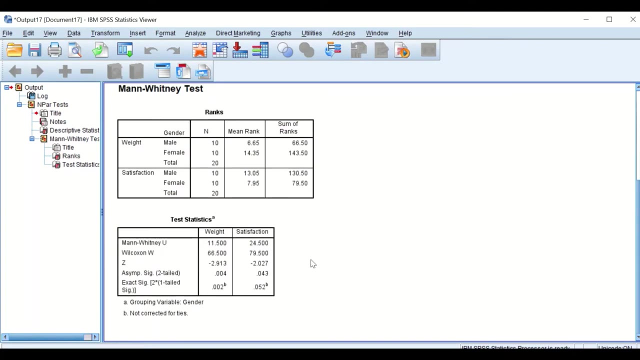 One's variable is the weight, the other variable is the satisfaction And, as we can see here is the female Rank for weight and male The rank also mean rank for satisfaction. Now, this is the most important part of the analysis here, and outcome. 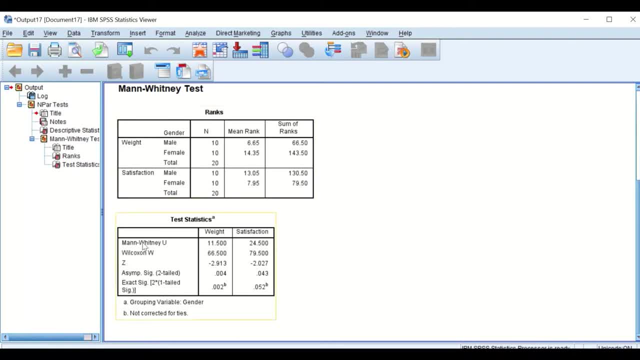 As we can see here, the man with new test has been calculated for both weight and satisfaction, And Wilcoxon also. And the most important part is the significance, As we can see here, this analysis showed that there is a significant difference between the male and female in terms of weight and satisfaction, because the p-value is less than 0.05.. 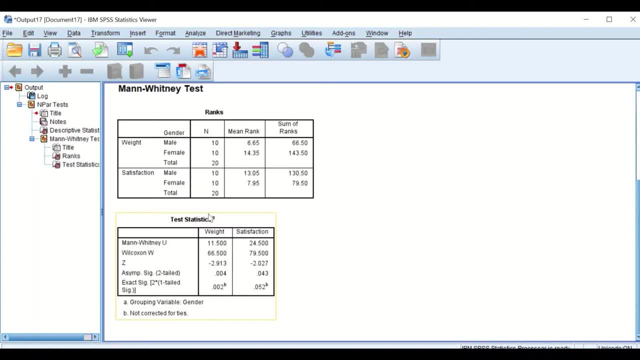 And this is considered to be significant. So there is a difference between these two groups, male and female, in terms of their weights and in terms of their satisfaction. So this is the way to do it. This is the way to do a man with new test. 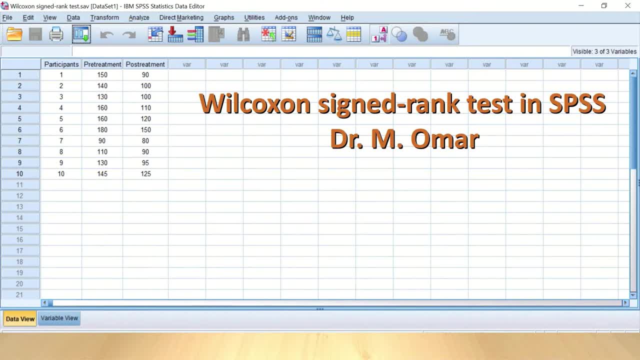 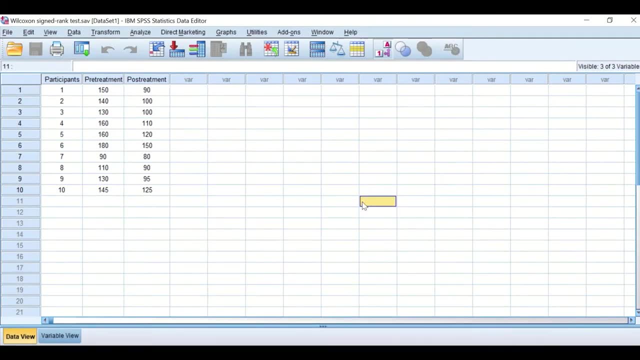 The second test is the Wilcoxon signed rank test. I have here a pre-entered data on 10 patients, So I have patient 1 to number, 1 to number 10. And they have been treated with a drug. This is the number that is really relevant to the cure of obesity and reduces the weight. 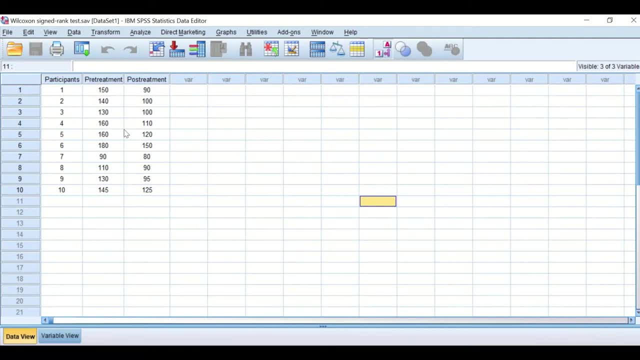 And then these numbers are the weight of the individual before taking the treatment and the column after and the post. And then the next column is the weight after taking the drug. And, as we can see here, weight does vary. It does vary pre- and post-treatment. 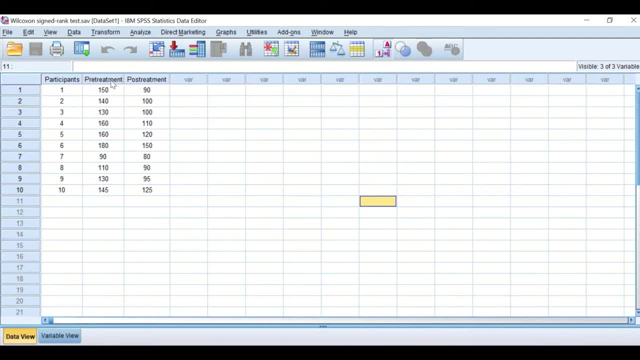 So we need to see where there is a compare, a difference between these two conditions- pre-treatment and post-treatment- on the same individual. So it's the same sample per sample, same patient before taking the drug and after taking the drug. 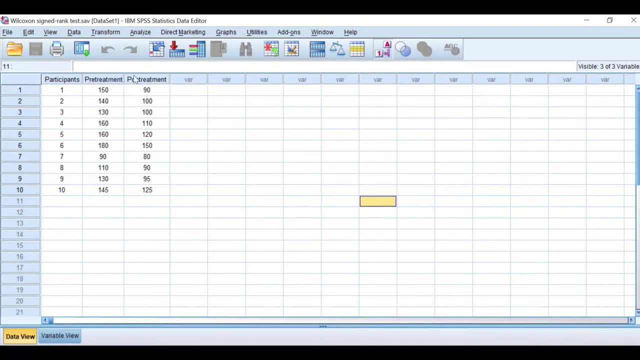 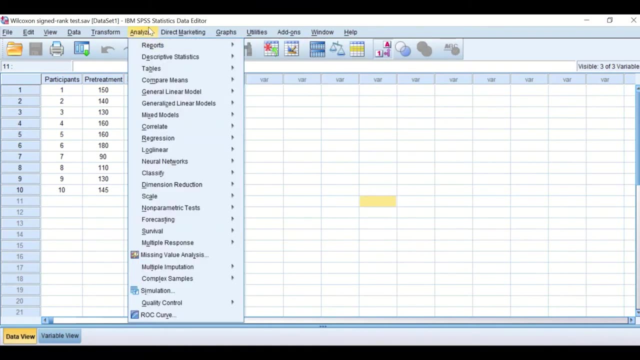 And looking at the effect of the drug, whether the drug is really effective in reducing the weight of a person, And for this data we need to use Wilcoxon signed rank test. To do that, we click on analyze. Scroll down to non-parametric test. 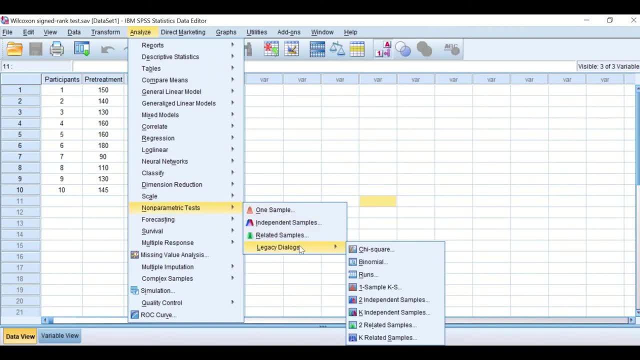 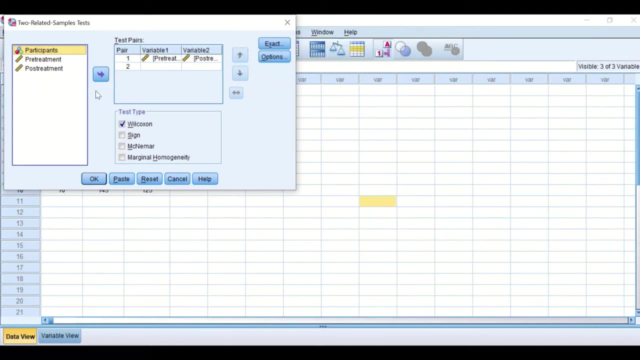 And then scroll click on legacy dialogs And then scroll down to two related samples. Here we need to use the two related because these samples are related. Another window will appear And in this you need to fill in a way that which two variables you want to compare. 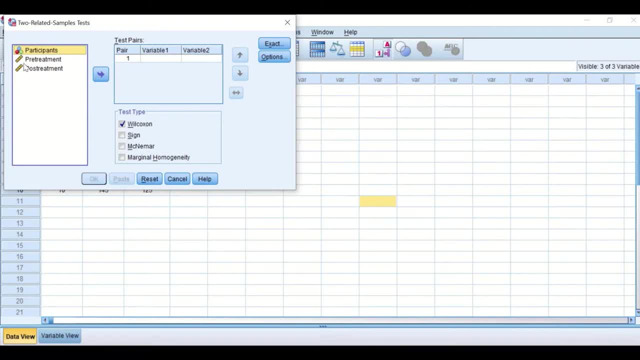 We need- let me do a reset for it. So we need to transfer the pre-treatment to the variable one and post-treatment to the variable two. So we need to compare these two variables to see if there is any significant differences between them. 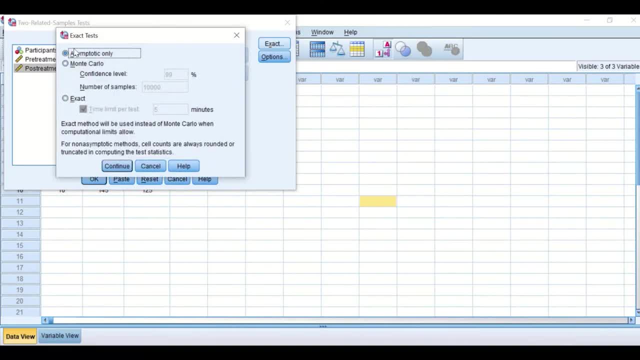 If we click on exact, I will keep asymptomatic only as it is And do nothing. at the current stage I will not use Monte Carlo, nor exact. Probably in subsequent video show you how it's significant, what's the difference? But we will stick with asymptomatic only. 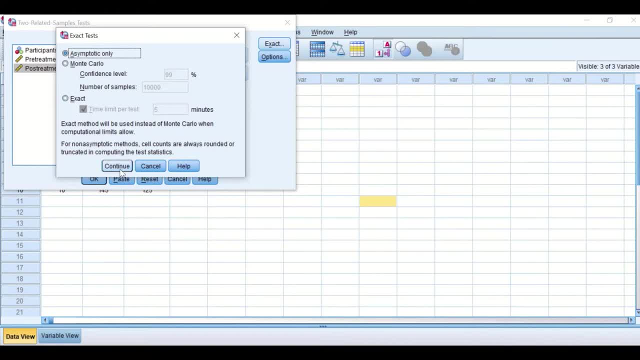 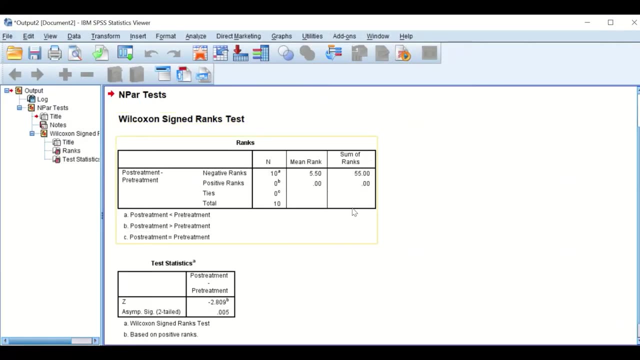 Asymptotic And then click on continue And then click on the Wilcoxon Wilcoxon icon here And then click OK. Now this is the output of SPSS. It's telling you that you have 10 samples. 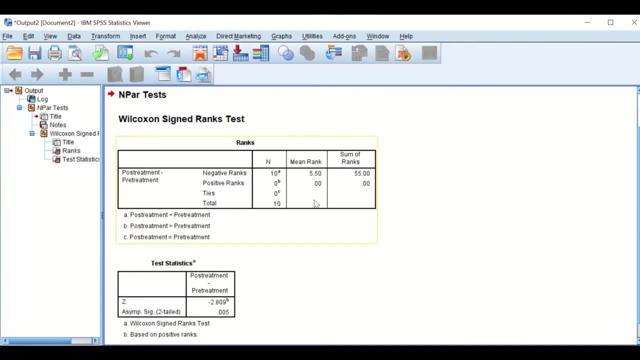 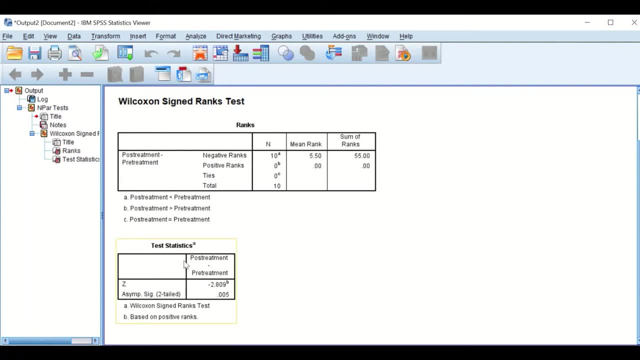 And they have been put in a rank And this is the rank for it: 5.5.. Now this small table here is the finding for the statistical analysis. This statistical analysis we're using Wilcoxon signed rank test. It's saying that there is a significant differences between the two conditions, as the p-value were below that 0.05.. 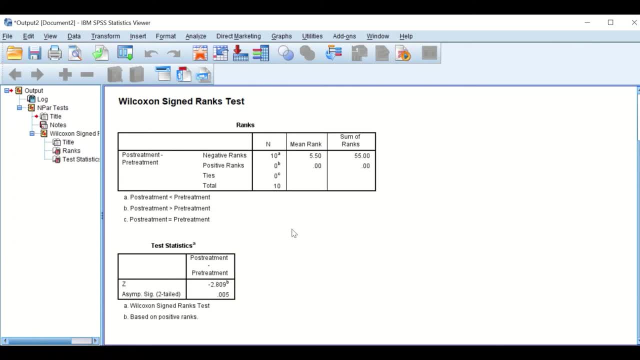 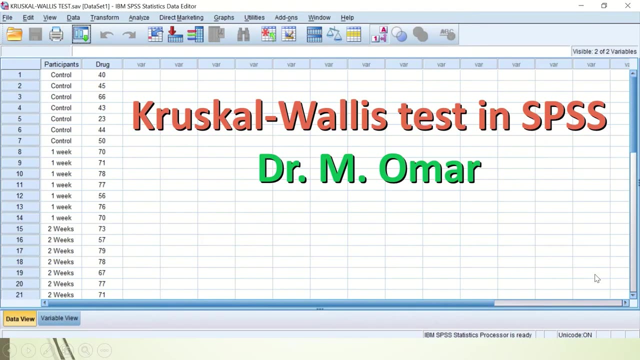 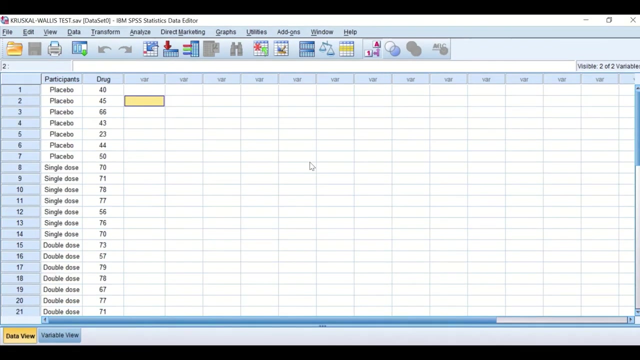 And so this is the way to do. Wilcoxon signed rank test on a sample that has two measurement that are paired measurement, ie the same person has been subject to different treatment. The third test is the Crescal-Wallis test. In data window I have generated really here a result or data in which in this data, I had really 21 participants in a study in which a new drug has been produced. 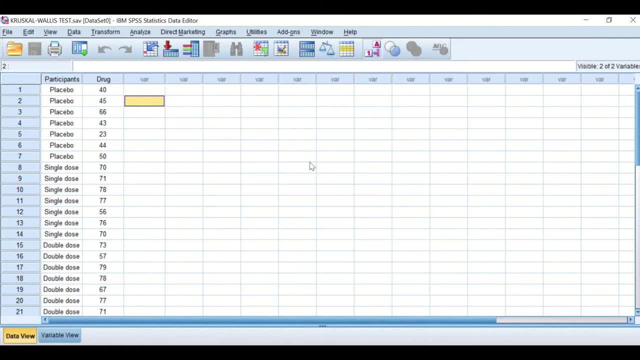 And I need to test the efficacy and effect of this drug on the sample. And I need to test the efficacy and effect of this drug on one of the variable, in effect on one of the plot component: the efficacy of it. So this group has been divided into three. 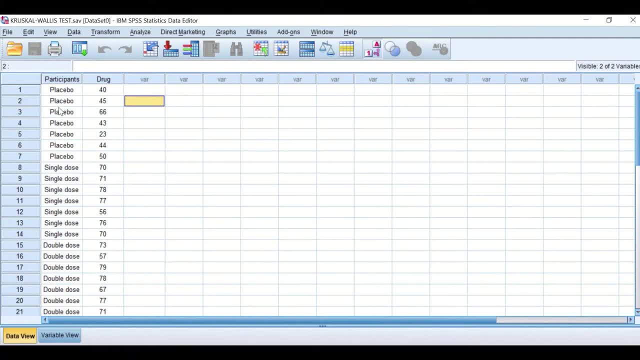 The first group has been given a placebo which is really not a drug- anything like water or salt and so on. The second group just giving single dose of the drug. The third group given a double dose of the drug And then the drug efficacy was measured. 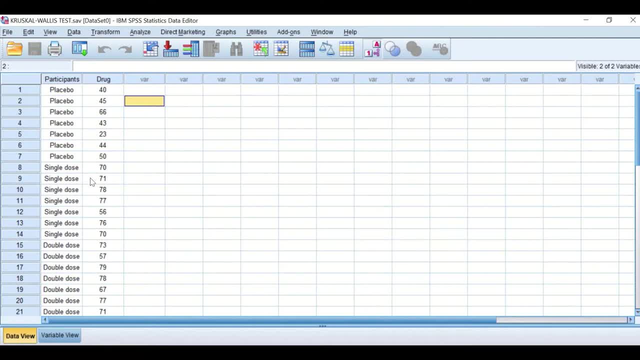 As we have seen here, through number given a number. So, as we can see here, the group size is small. All the groups are seven in each group of seven participants And I've checked the distribution of the data in the drug section or variable, and it was not normally distributed. 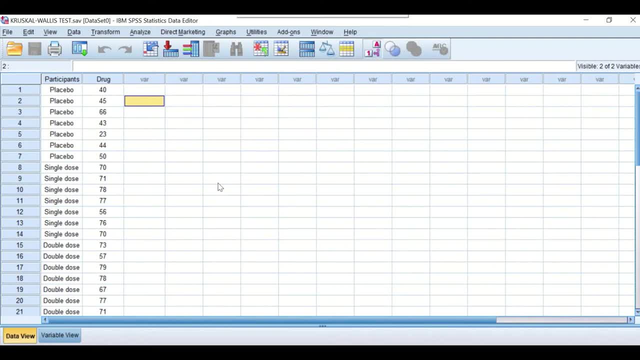 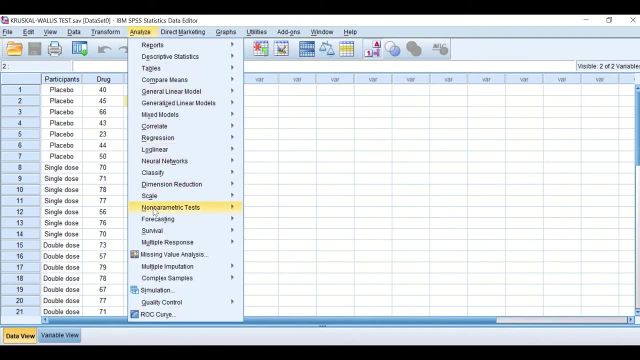 So how can we really calculate? How can we calculate the significance of the drug? So let's look at the distribution of the data between these groups. OK, The way to do it is to click on Analyze. Scroll down to the nonparametric test, because this is nonparametric data. 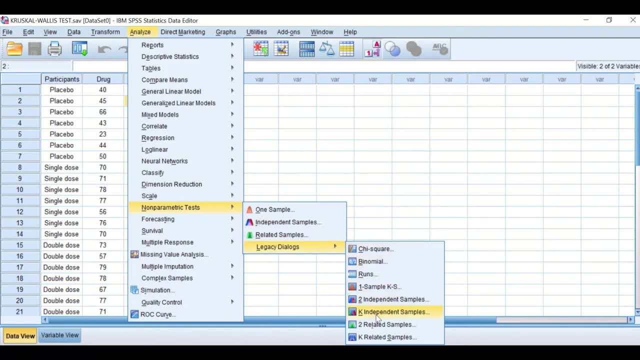 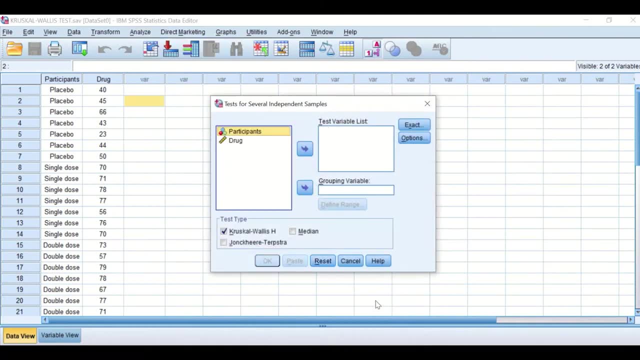 And then click on Legacy. Then scroll down to K. Individuating K indicates that more than two samples. Click on that And then reset that. Another window will appear. There is a test type called KSKL. We'll click on that. 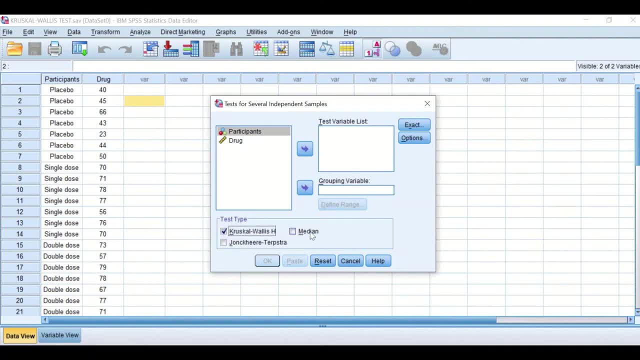 So we need the KSKL, KSKL 12S test. We'll transfer the drug into the variable list to test the variable Participant. we will move it into the group variable And in the group variable I'm going to tell the software. hey, listen, I want you to look at the group from number one. 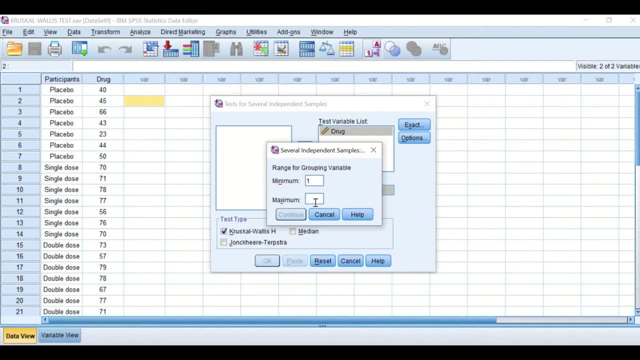 Number one. I give it. It has been assigned for placebo to maximum Number three. Three is from one to three, So the placebo, single dose and double dose, And then click on OK. Continue For the exact link. look in the exact test. 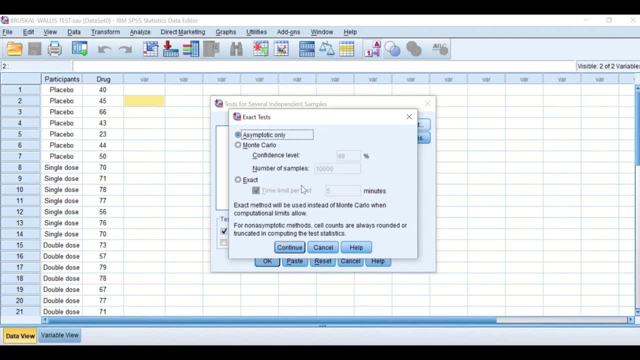 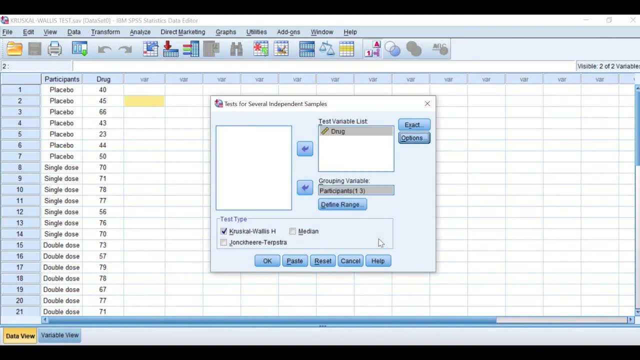 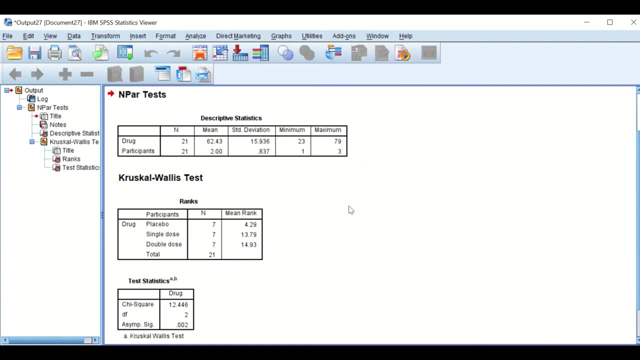 We'll just give it asymptotic only, And then the options: I will select descriptive And then I will click on Continue, Then hit the button for OK And then an output SPSS Window will appear telling you the drugs has been part. 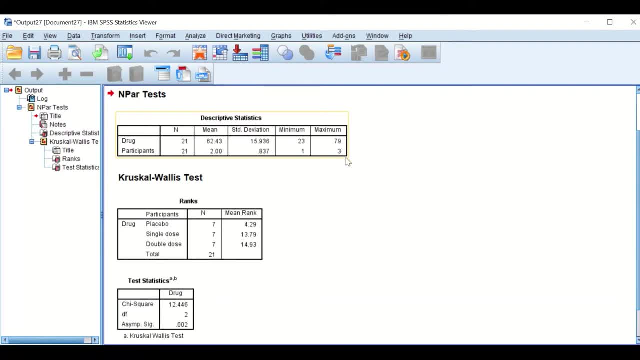 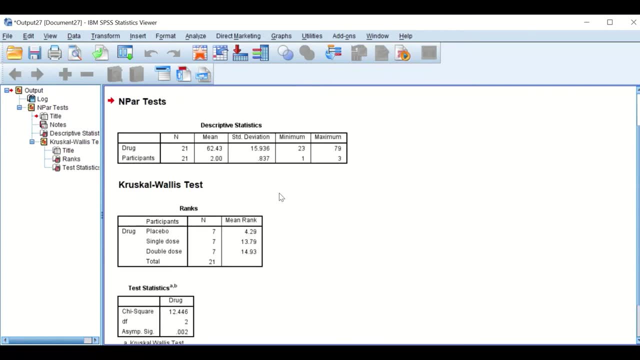 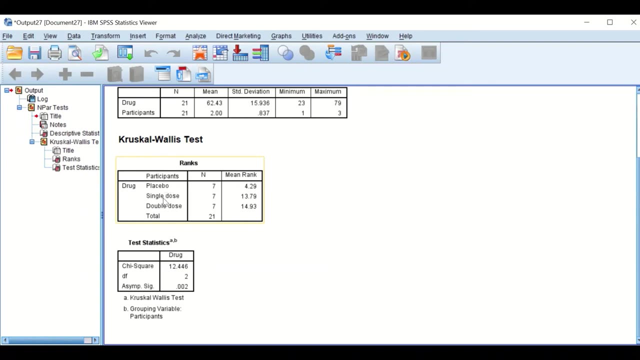 There are 21 part participant on this study. It will calculate the mean and the standard deviation. However, what's important as this is descriptive data, Wall, KSKL, Wallace test. As we can see here, three groups: placebo, single dose, double dose. 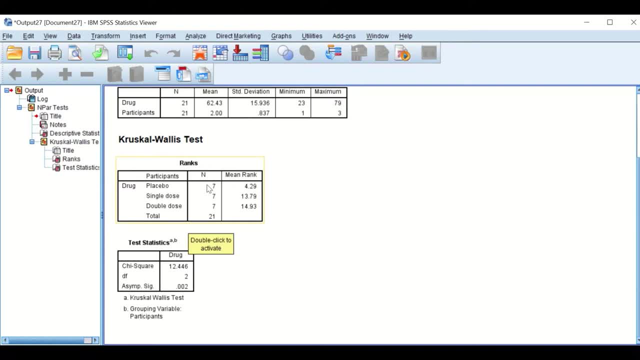 And again, as you can see, there are seven participant individuals in each group And if we look at the again, that KSKL ignored the value of each Number in the drug and rank them didn't work in the actual data. It took these data and rank them and put them in rank and give it a rank. 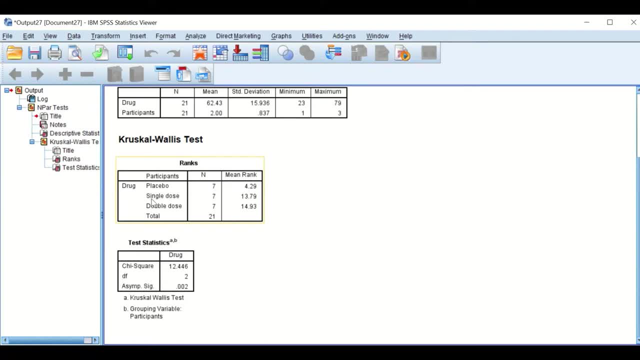 So the mean rank for the placebo is 4.2 and for single dose 13 and for double doses 14.93.. As we can see, there is a difference in the mean between Placebo and single dose, placebo and double dose. 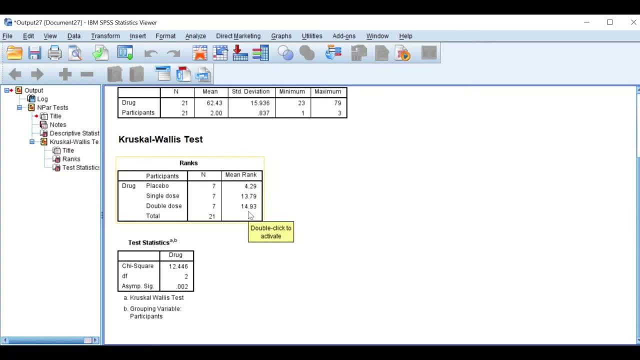 But there is nothing, no difference, not significant, not that much difference, Let's say, between single dose and double dose. Now KSKL Wallace tests in SPSS has calculated the overall significance and comparison between these three groups And found out there is a significant differences between these groups. ie taking the drugs make changes. 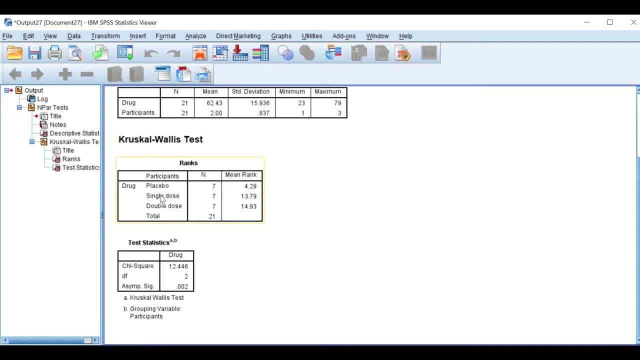 But doesn't specify Which two groups are significant and which are not significant. As we can see here, the mean rank between single dose and double dose is very close, So if I want to find out which groups really giving a difference, it has a significant difference. 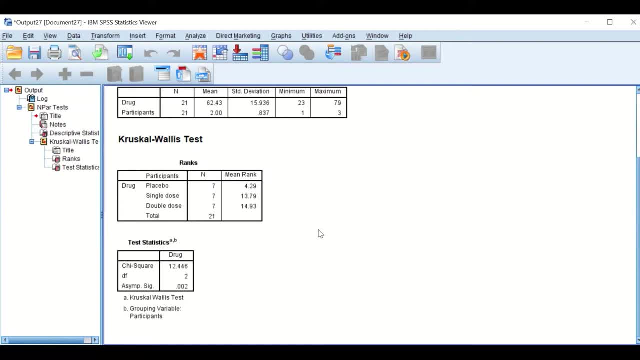 Specifically significant difference or effect of the drug. We need again instead, in addition to do KSKL, to go back again and do Mann-Whitney-Yu test for placebo and single dose. placebo and double dose, Then single dose and double dose. 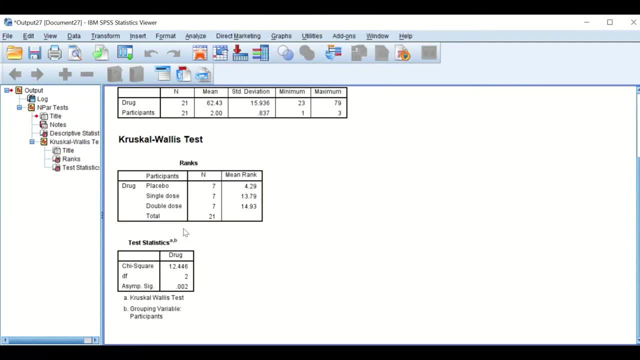 And I will show you already how to do it. I've already shown you how to use Mann-Whitney-Yu test in a previous video clip. You can have a look at it. But the way to do it is to go analyze. 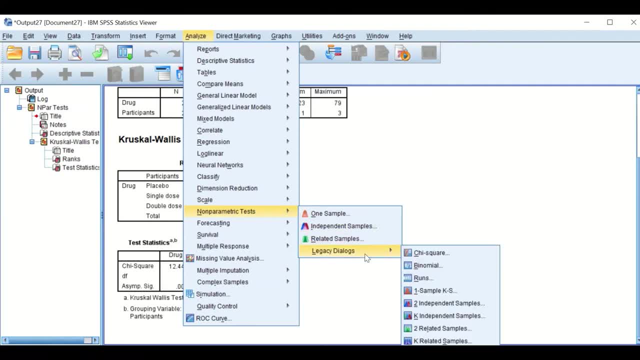 Click on non-parametric again And then click on legacy dialog And then we need to click on two independent, Because these data we have are independent. So we click on that. Reset that Again, Again, And I need to click here on Mann-Whitney-Yu test. 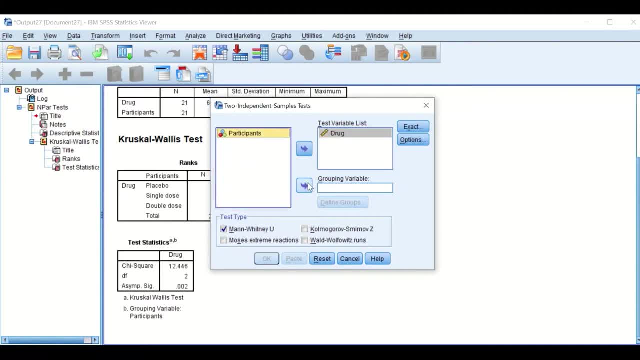 I need to put the drug in the testing one And the participant here And I will come, And then I want to define the group. Here we need to test, compare, test two groups together. So group number one is the placebo type one. 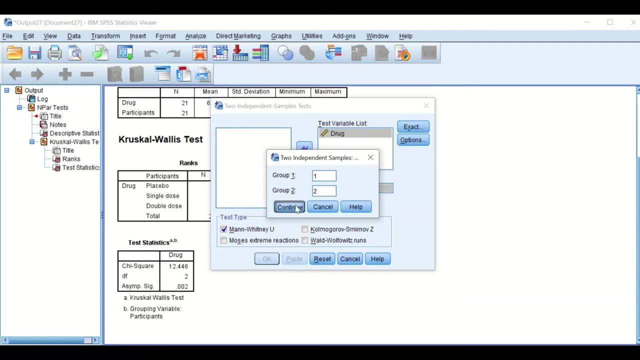 And group number two is the first single dose. Click on continue. Exactly, We'll leave this window as exactly the same For option we'll take. only click on descriptive, And then we'll click on continue, Hit the OK button And voila. 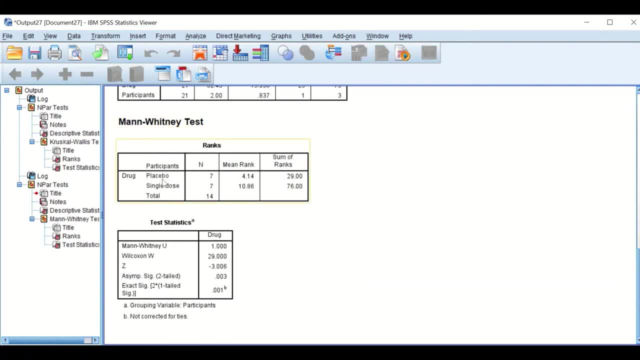 We see here that the Mann-Whitney-Yu test has been calculated for placebo and single dose And it was found that there is a significant difference, that if you get the first dose of the drug, you get really a difference between control, placebo, which is a control, and the single dose. 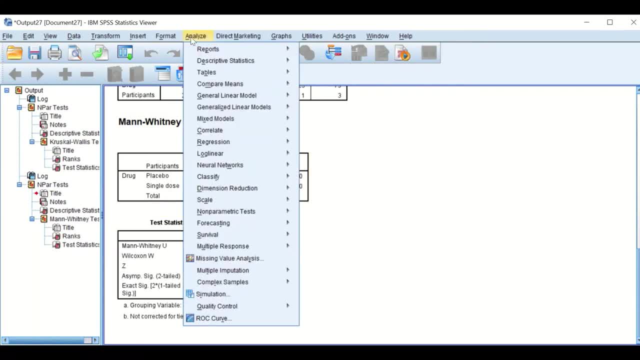 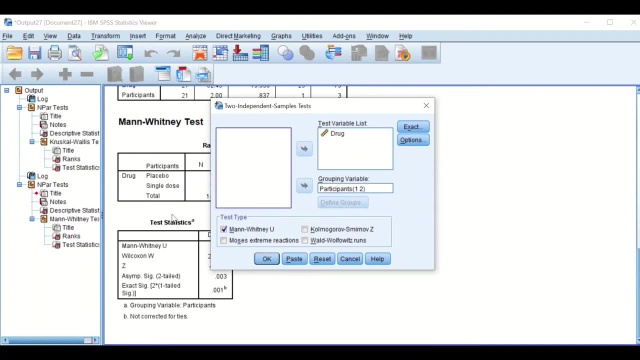 So there is a significant difference. Now let's see if there is significant difference between Between placebo and double dose. So we'll keep. group one is the placebo. Group three is the double dose. Click on OK. Keep everything, and click hit OK. 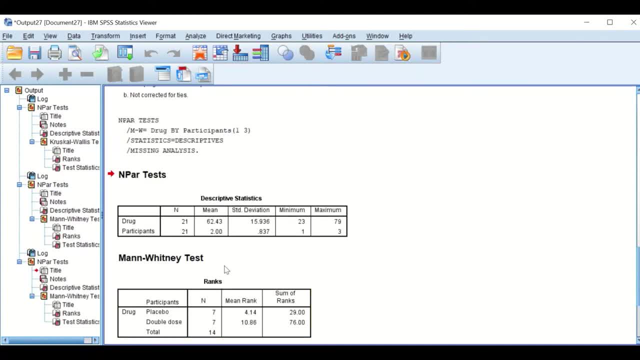 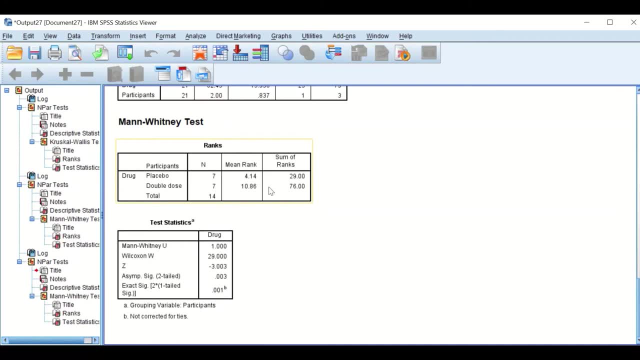 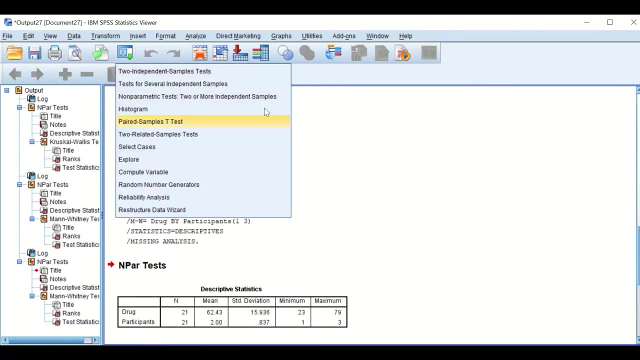 Again. we can see that in this, in this test, In this test, the value is again is also 0.1 between placebo and double dose Of the drug. Now, if we again go back again and we do also The same test, but instead of comparing one to three, we click on two to three, 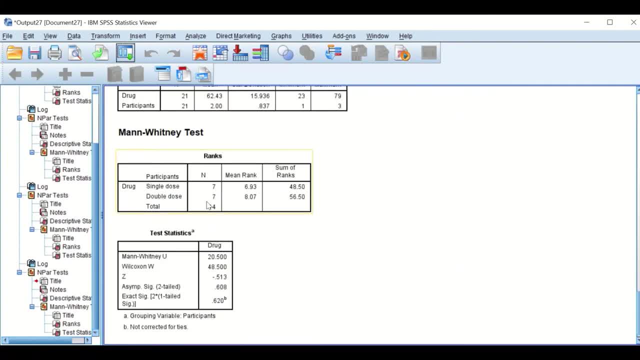 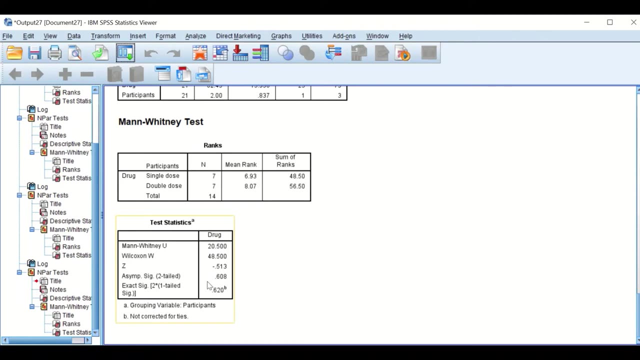 Click OK, Keep everything the same. And again, Mann-Whitney-Yu test has calculated this difference, calculated the significant difference between single dose and double dose And, as you can see here, there is in fact no differences between the single dose and a double dose. 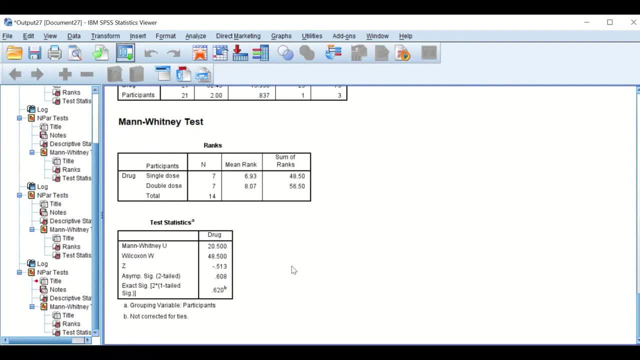 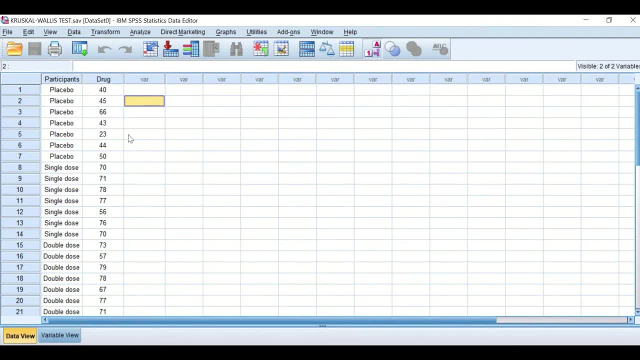 This p-value was 0.6.. From this data we can really show that has shown that CARES-Cal Wallace test- that tell you that there is a difference, significant difference, between all these three groups, But it doesn't tell you which group with which group has really significant. 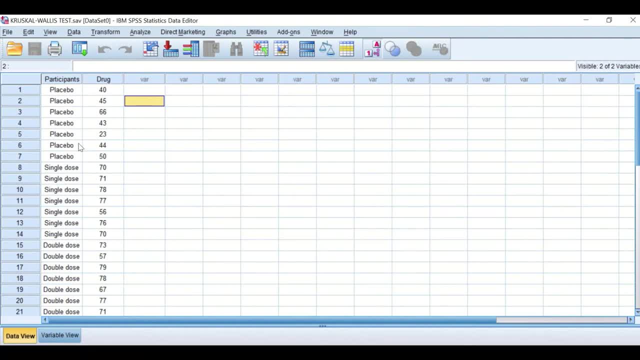 We have found out that placebo with single dose is have a really significant difference, Placebo with double significant difference. But once we compare the single dose with a double dose we couldn't find a significant difference. That's indicate that giving a pair an individual single dose or a double dose will have the same effect compared to placebo. 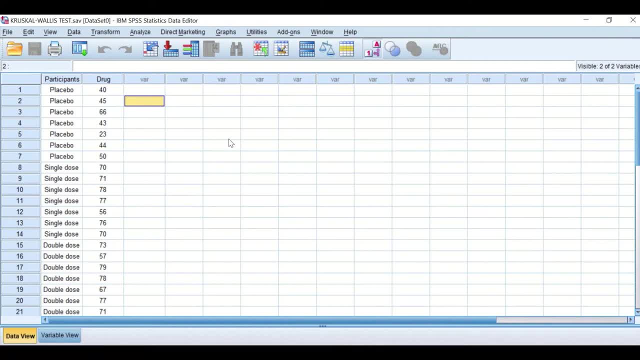 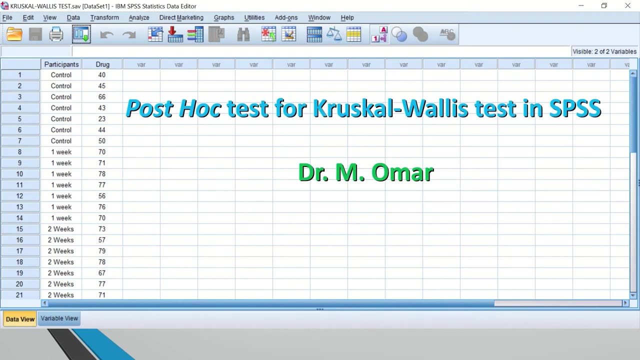 This is the way to do CARES-Cal Wallace test and then to do a subtest to determine which of the subgroup that have really statistically significant. Post hoc test is another test that is done following the CARES-Cal Wallace test, Just as a complimentary for the test. 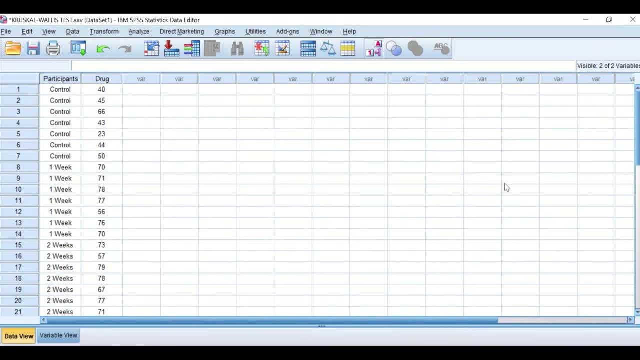 In this data view I have three group: Group number one, which is a control, Two is the one week and three is two weeks. So these three groups are drug. New, novel drug has been designed and its effect has been followed up using 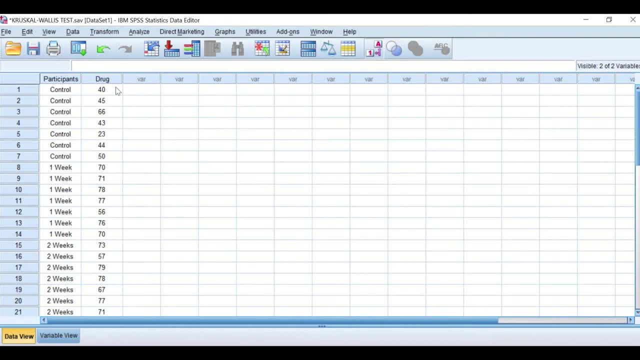 Specific parameter in the blood. So we want to compare the efficacy of the drug After using it for one week and two week compared to a control. Again, I've double checked the distribution of the each group control, week one and week two, and they are not normally distributed. 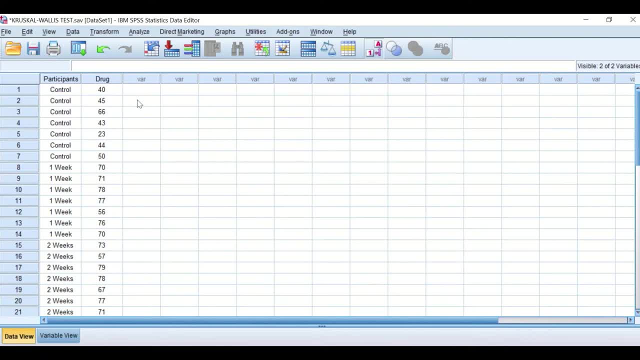 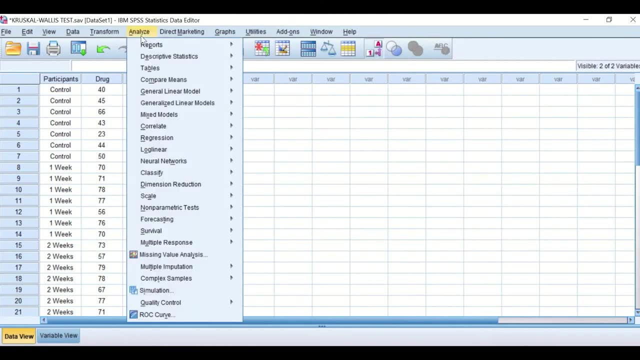 So how can we do CARES-Cal Wallace test to determine the significance, Whether there is a difference in significance between these groups? Click in analyze, Scroll down to nonparametric test And then to legacy dialog, And then we click in the on the icon for K independent samples. 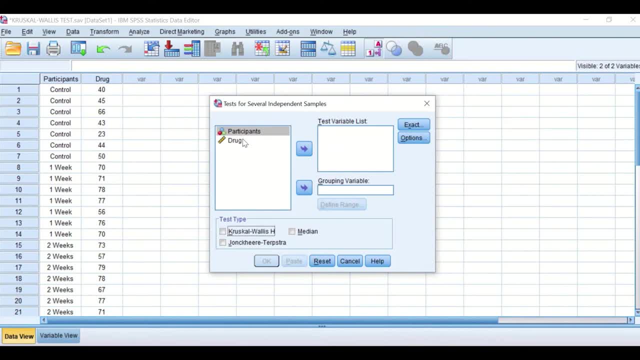 Reset this. Okay, so I'm going to transfer the drug into test test variable list And the participant into group variable And in the participant I want the range to be from group number one, in which I gave the control value one, And to the week two, which is value three, and week one is value two. 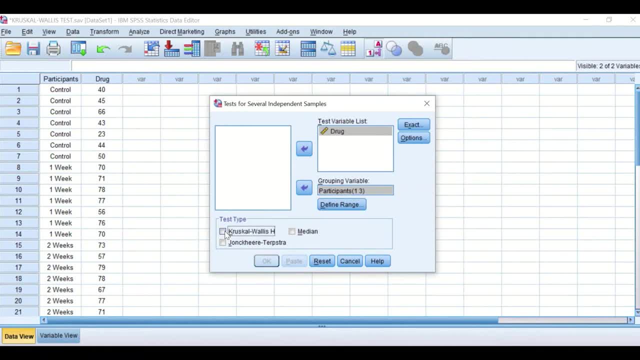 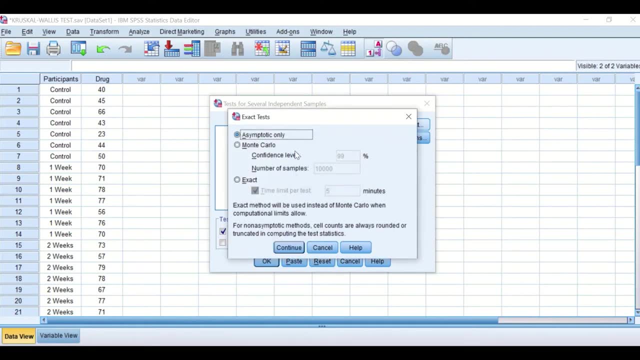 Click on continue. Click on the icon for CARES-Cal Wallace And then check on. click on exact. We'll leave. our new window will appear. We'll leave the asymptomatic only test as it is. Click continue on the options. We will just click on the descriptive. 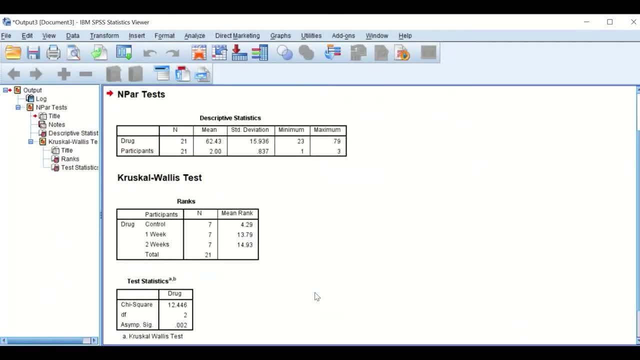 And then we click continue. Hit the button for okay. SPSS will produce these tables. As it says here, 21 participant involved in this study And out of these 21, seven were controlled. Seven week drug has been given for one week and two week or two weeks. 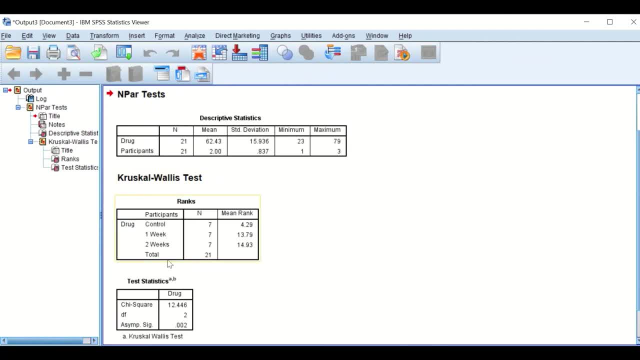 And what has this CARES-Cal Wallace test done? is put took the actual data for each one of these and sort them into ranks and then calculate the mean rank And we can see from the mean rank that control compared to week one week is. really there is a huge difference from 4.2 to 13.. 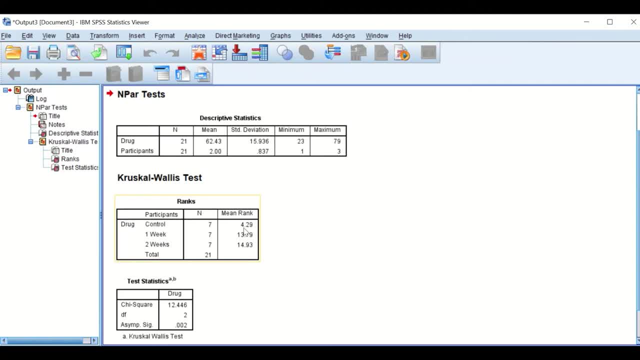 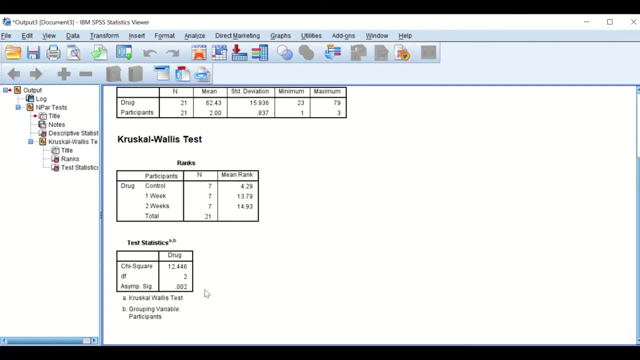 And from control to two weeks is 14 or so from four to 14.. However, there is no big difference between the mean rank of week one and week two. The test produced a significant value, P value, And the P value is lower than 0.05.. 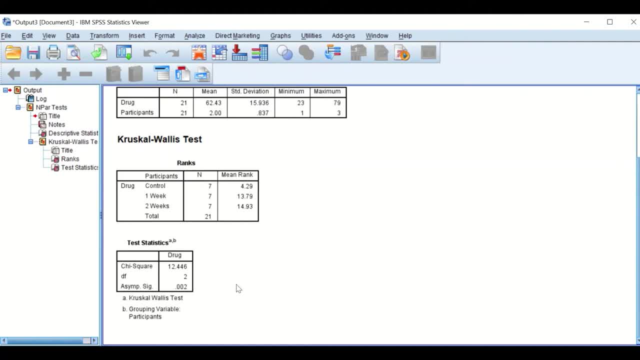 Which really indicate that there is a difference between patient or individual participant who has taken the drug for a week compared to control, or two weeks compared to control, And but it doesn't tell you if the difference where there is a difference, significant difference, between the control and the week, or the control, week one or week two, or week one or week two. 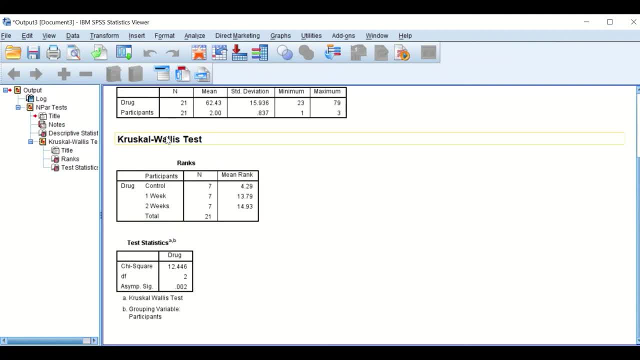 It's just give you a P value for all three groups. And now to nail down this, into which groups. which two groups really are? See, They are significant, which are not. As I see I showed you in the previous video clip, can go and do man with me. 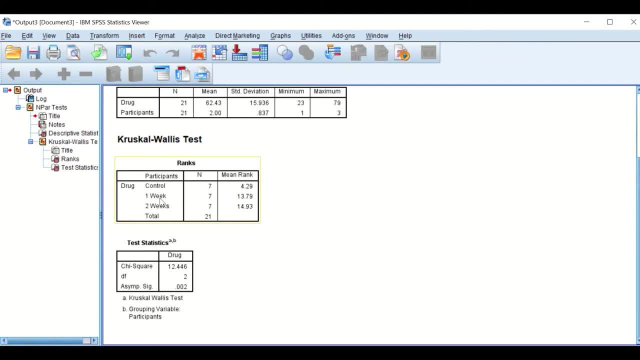 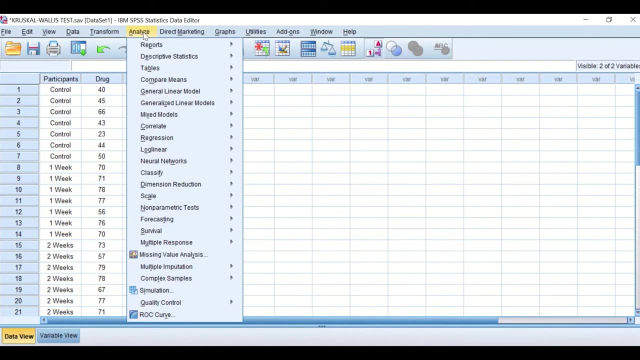 You test on two samples: control and week one. control and weeks to two weeks and weeks one and week two. However, there is another way to do it, which is called post hoc test. to do a post hoc test, I'll go click on analyze. 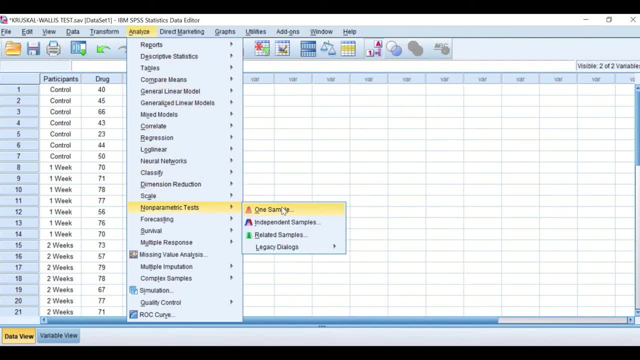 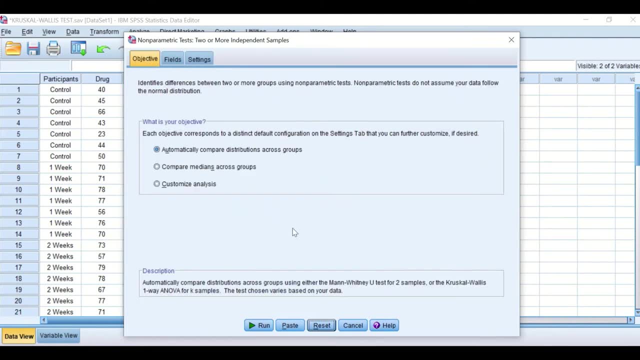 Scroll down to nonparametric test. Click on the independent samples, Click reset here. Objective. So in this icon, in this window, I will appear and ask you: what is your objective? Say: I want to customize the analysis, I want to tell the software what to do. 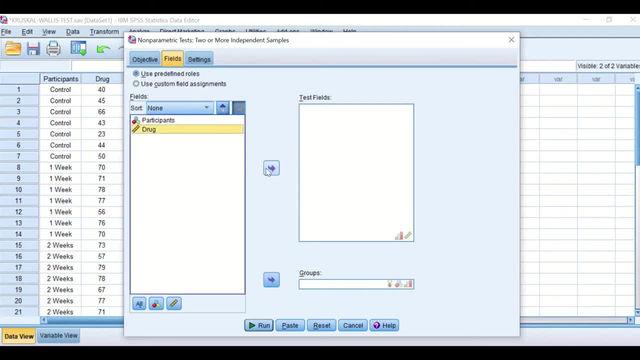 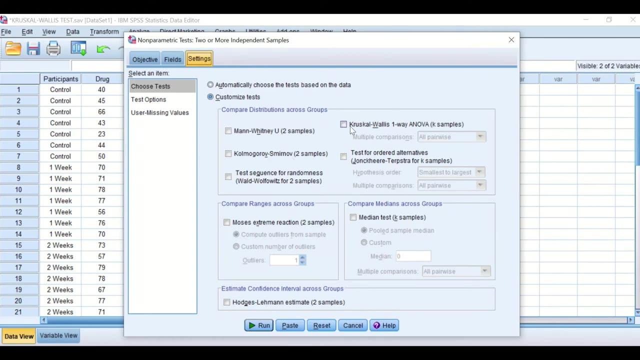 Click on there in the field, I'll transfer the drug into the test field and the participant into the groups And then in the last Icon here is the settings. So what I want to sort to the sitting. I will click on customize test and I will click and care scale Willis one way. 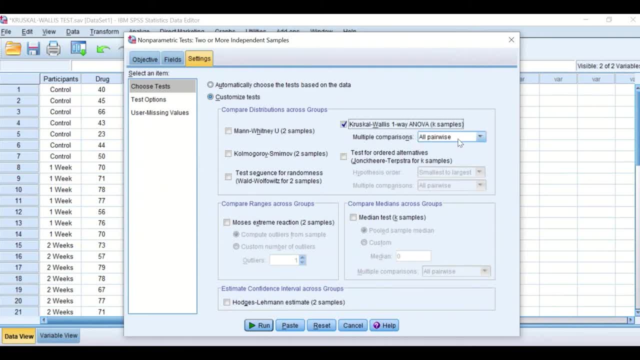 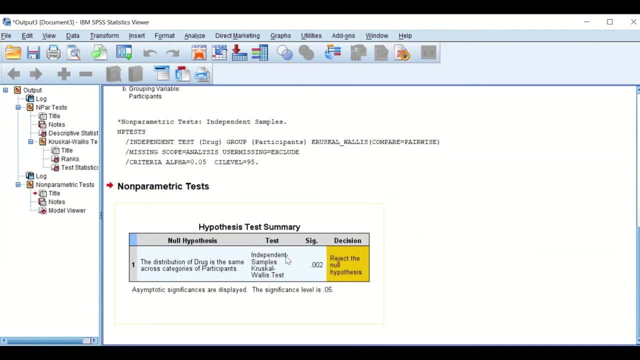 And it's automatically says: do multiple comparison pairs all pair wise? So it will do a pair wise between control and week one, control, week two, week one and week two, weeks two together or two weeks together. So I'll hit the run And then a table, small table, saying here that the hypothesis test, testing that there is a difference between the three groups and the difference is point 002.. 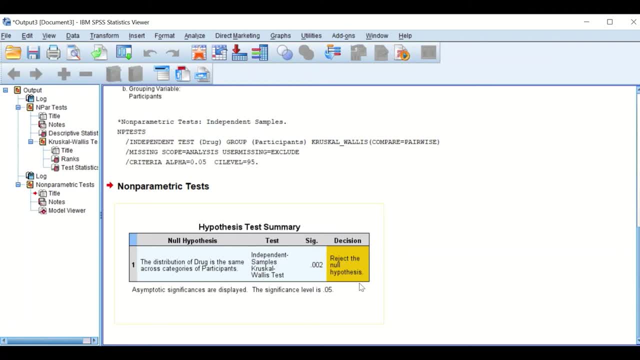 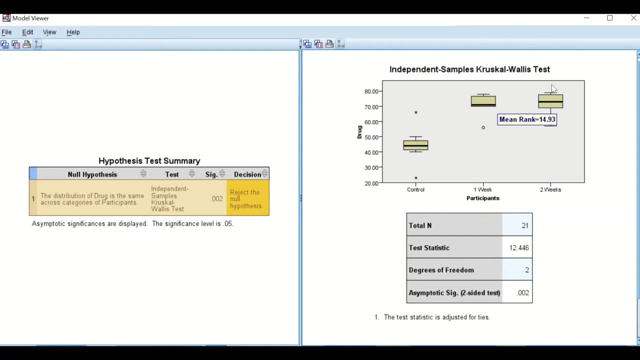 And to find out which groups, which two groups, really have a significant value and which are not. Double click on that. Okay, So I'll hit the run, And then another window will appear showing you the box plot for control: one week and two weeks. 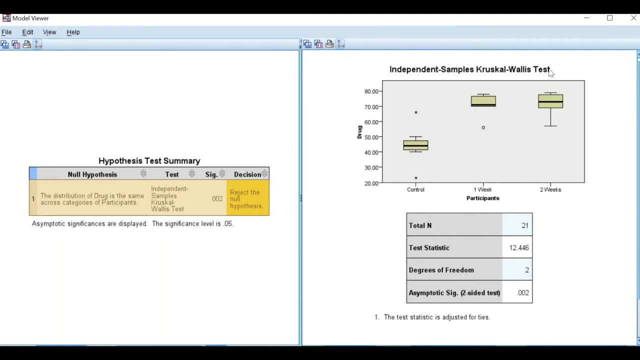 As you can see, there is not that much difference from this diagram between one week one, one week and two weeks, But there is really a difference between controls and week one and week two. weeks to do, to do, And then we click in another one called pairs wise. 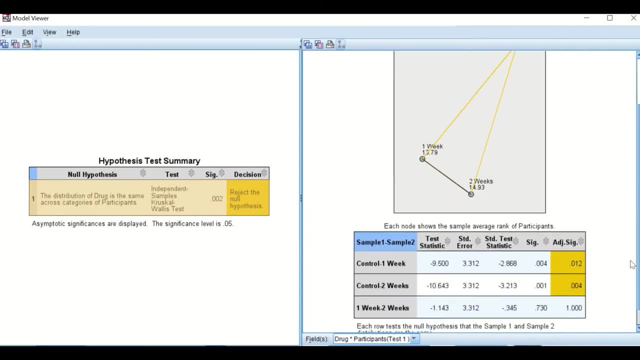 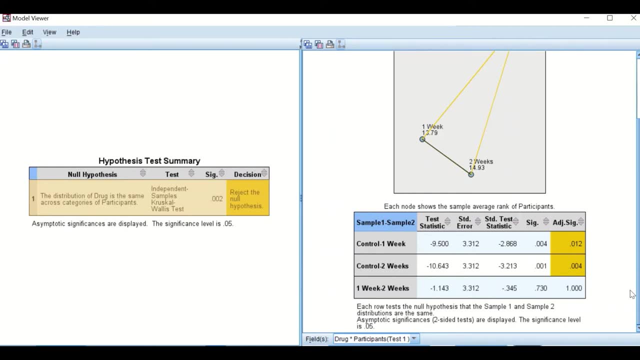 Comparison- That's a table- will appear here. That's the table that will really do that comparison of control one and week one week And it's give a significant value of 0.012.. When a test has been done to between control and week two weeks, it's less than 0.05 significant. 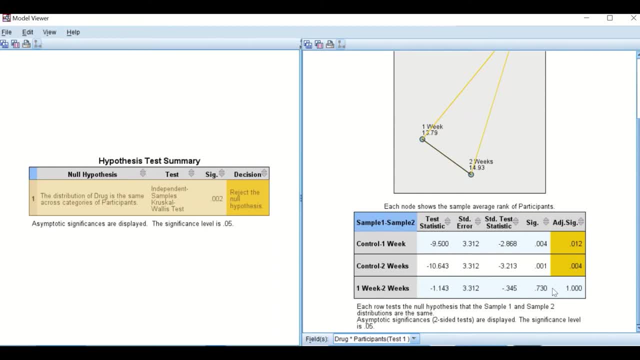 However, when we compare week one with week two, there was no significant. The value was one. So this table is tell you, Can Chris Kerwallis tell you that there is a significant difference between all the three groups. This table, both hoc test, will tell you that control and week one is significant control and we two weeks significant. 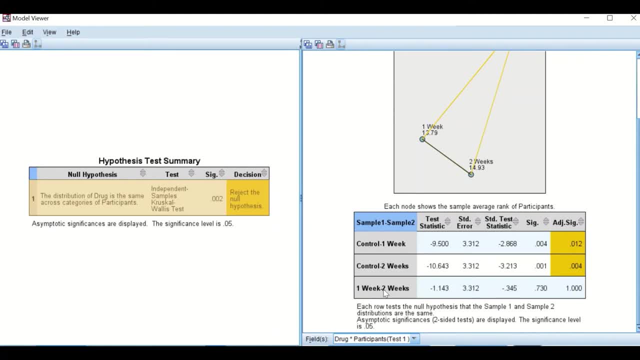 However, there is no significance between week, one week and two weeks. So from this data we conclude that a patient giving this drug or individual given this drug Taking it for one week is more than enough to have an effect, As two weeks and one week effect is nearly similar. 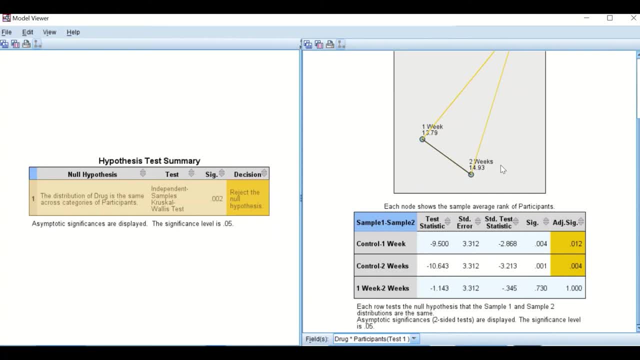 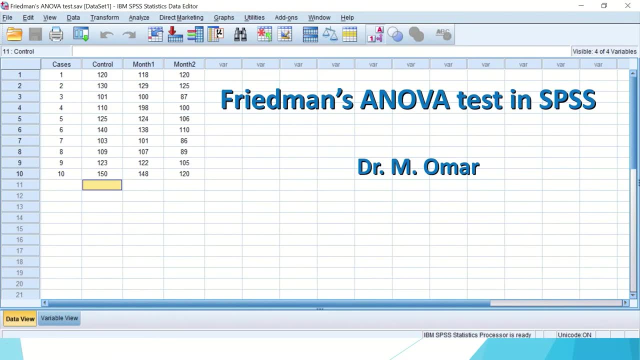 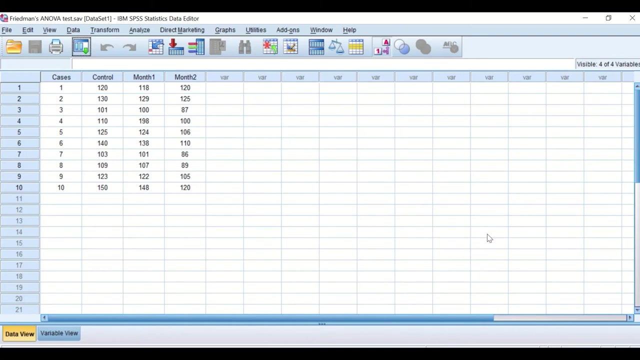 This is the way to show you care scale: Wallace test, followed by post hoc. The final fourth major nonparametric test in SPSS is the Threadman's ANOVA test. This is a data taken from ten participant in this study. Participant one to ten. 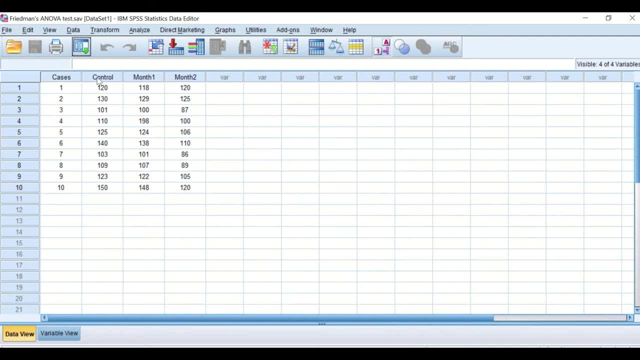 And a body weight was measured at specific point at time. on that study, The aim was to look for the effect of exercise on the body weight. So each individual body weight was measured at 0.012. Before the exercise And then body weight was measured at after one month of the exercise. 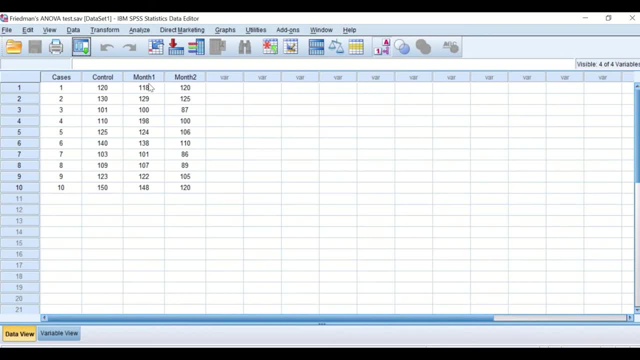 And the individual was doing a half an hour exercise, sport, per day And then at the end of two months or so months or so, the body weight was measured again. So we can see here from this data that each individual has a measurement. 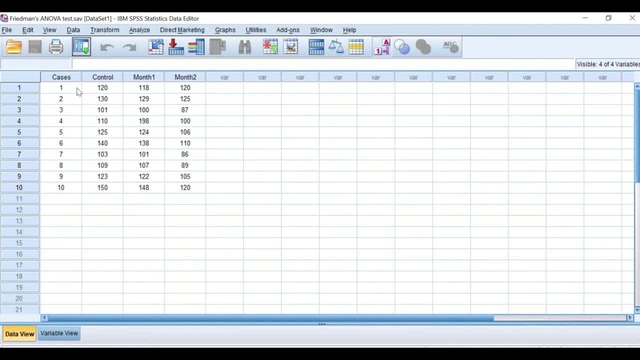 So these all Three columns are related. So these data are related And if we want to find out if there is a difference between all these three variables or samples, Since they are small- ten cases- and the distribution of that data on each group is not normally distributed- 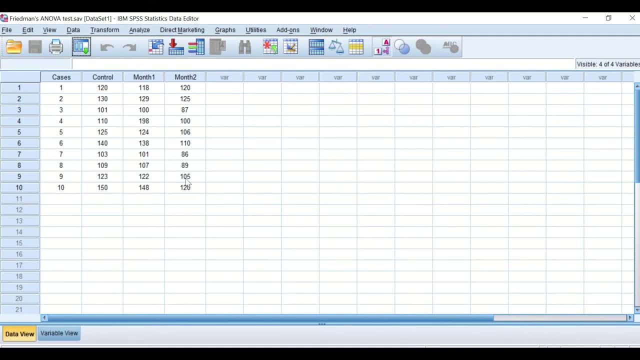 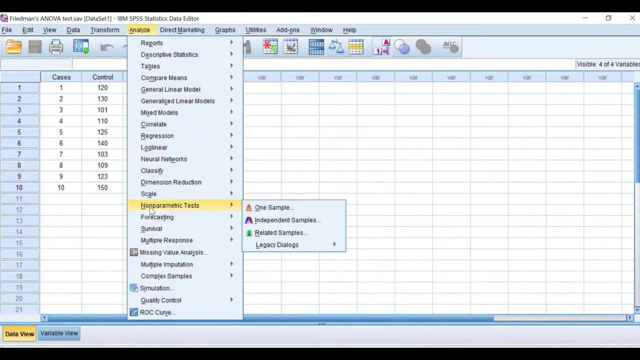 I have checked that and I will show you in a future video clip how to do that. So to do the analysis on these data- non-parametric and small and not normally distributed And more than two groups- We click on analyze. Go to non-parametric tests. 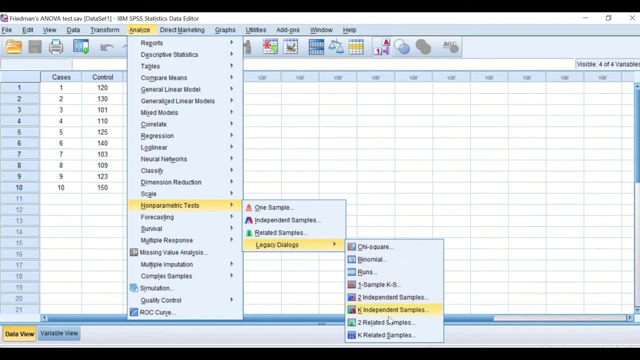 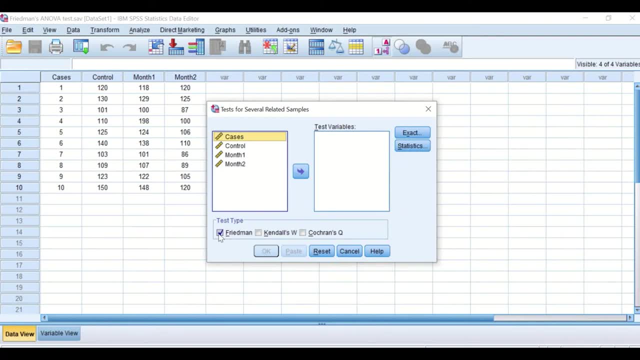 Then legacy dialog, Then scroll down to K related samples. Hit the button. You will have a window here asking you Again. as you can see here, there is an icon for Friedman Friedman tests. We will click on that. We will ignore this. 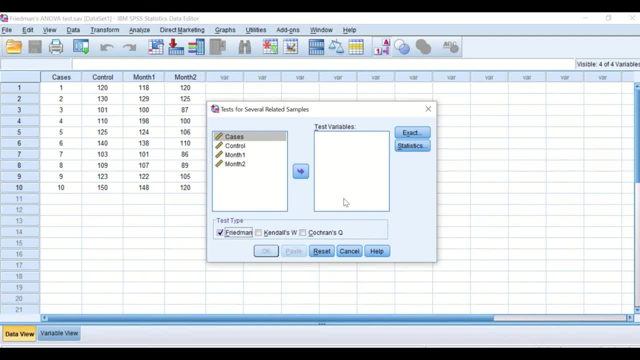 I might come to this later on, a subsequent video clip to explain the difference between all these three. So I want to transfer the control to the test variables and the one month and two months And I will click on the exact. I will keep this window the same. 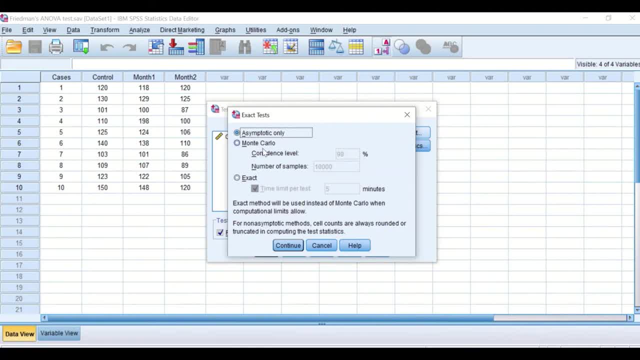 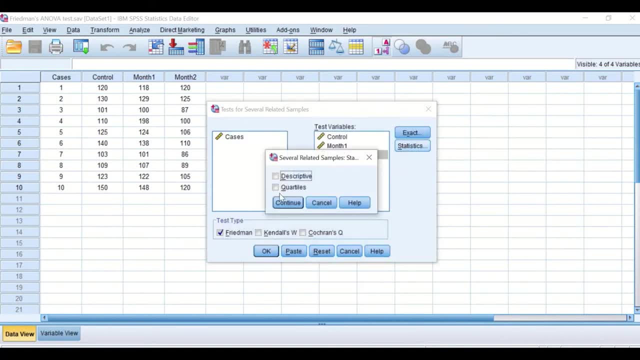 I will not do any further changes. I will explain in depth in future videos what is Monte Carlo and the exact Statistics. I will click on that icon and I will select descriptive and click continue. Then click hit the button for OK. Now SPSS will generate an output. 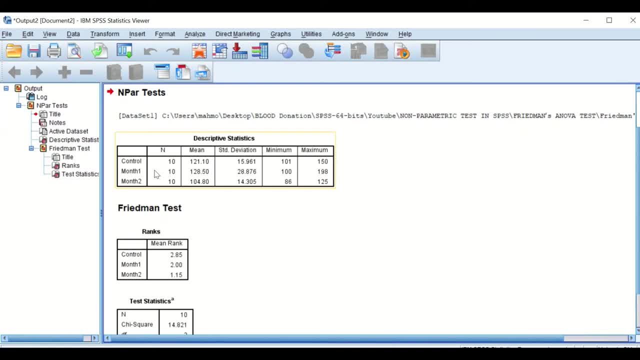 Will give you some descriptive statistics: The control, the one month, the two month, The samples in it, 10, and then it will work out the mean for each body weight in each group and the standard deviation. However, this is not of our concern. 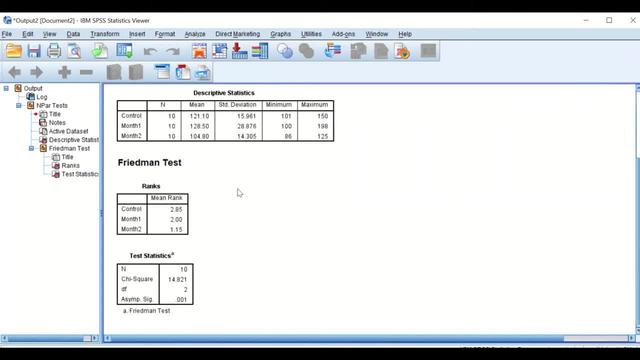 Our concern is really Friedman test. So what happens? So what have Friedman test did in this SPSS? It took the data from the control month and two months and put them into rank and worked on the rank and then calculated the significant difference between all the three, all between all the three groups. 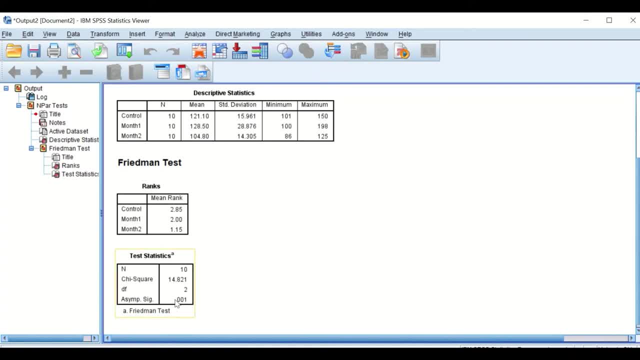 And again, the Friedman generated a p-value that is less than 0.05.. This data and these analysis, This test, shows that there is a significant difference between the three groups, But it doesn't So there is a difference if you exercise one month or two months, compared to no zero exercise. 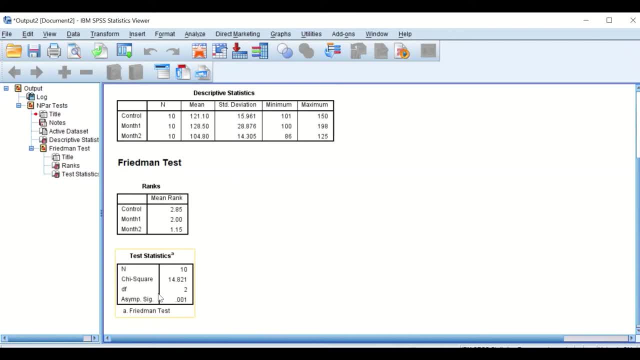 So. but that test doesn't tell you which which groups- two groups together- are significant and which are not. So there is, There are two way to do that. I think I will show you one in another video clip. I'll show the other one. 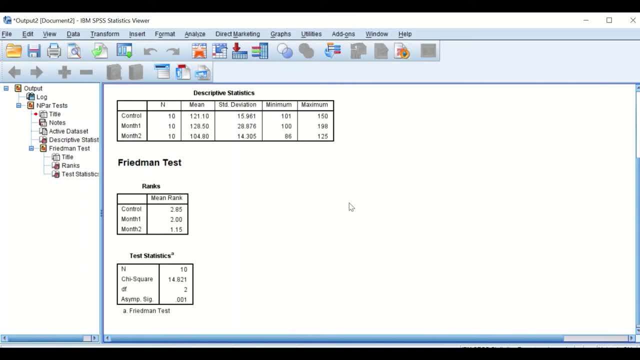 I'll show you another way. So there is one way. One way to do that is to go to do paired tests- Nonparametric paired test- and nonparametric paired test is a Wilcoxon signed rank test. To do that, we click on analyze. back again to nonparametric test. 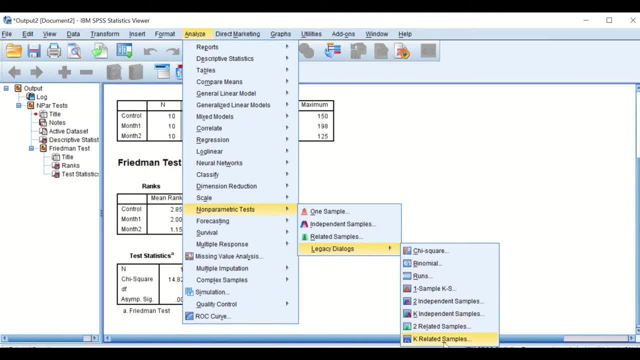 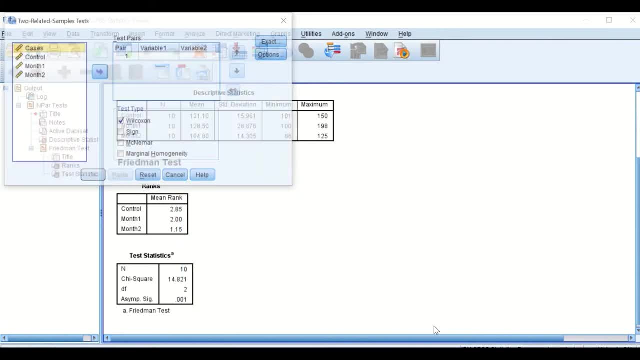 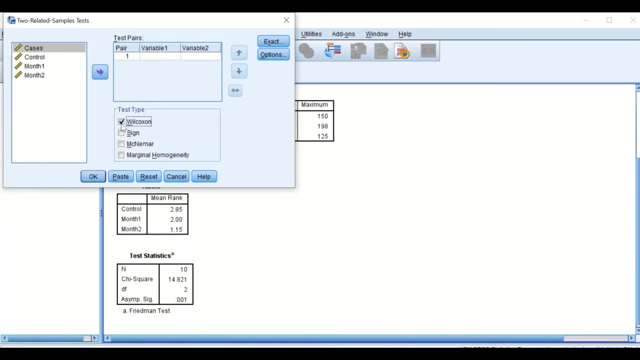 Then legacy dialogue, And instead of clicking K related for this, K for more than two samples, We'll go for two samples, Two related samples. A window will appear And, as you can see here, Wilcoxon test is. icon is clicked on. 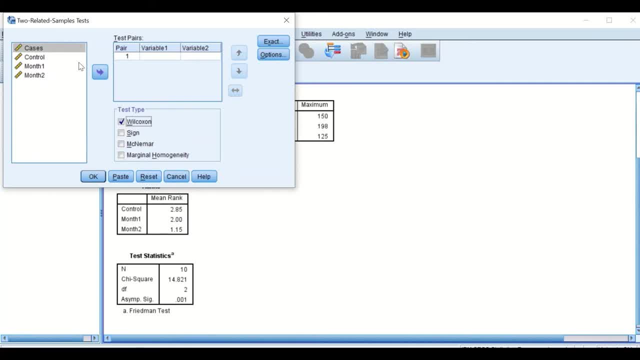 So what does this test do? Will compare the variable Between control and one month control and two months, and then one month and two months. To do that, we click on control and click on it. So, and then I want to control, to compare control into. 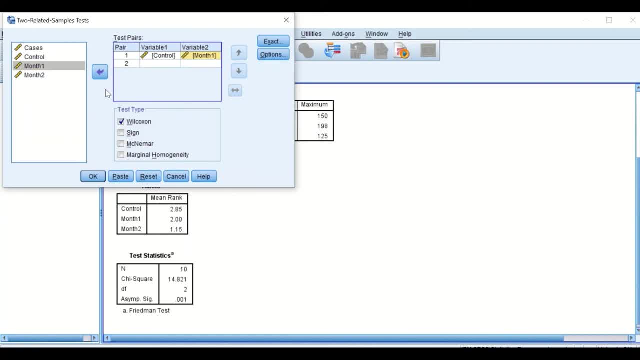 Month one. click on it. And then again I want to compare control to two months. Click on that, And then I want to also to compare one month to two months. So here now I have a combination comparing control to one month, control to two months, and then one month to two months. 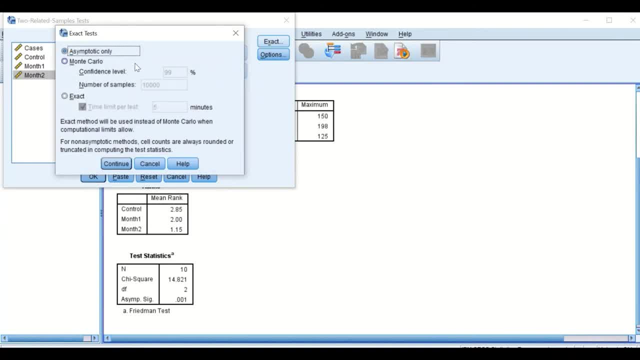 Here. I will click on exact And, as I can see here, we will just leave this window as it is And hit the continue On the options. I will click on descriptive And will I? I will click on continue and then I click OK. 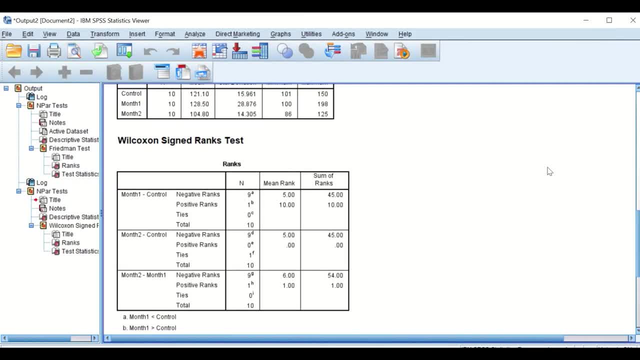 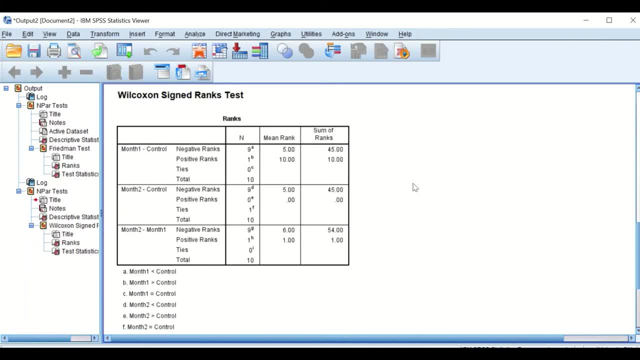 Now hit the button for OK. This Wilcoxon signed rank test is calculated And, as we can see here in this Wilcoxon, similar to Friedman, But the data take the actual data in two groups and put them in ranks and then compare the data in one month to continue. 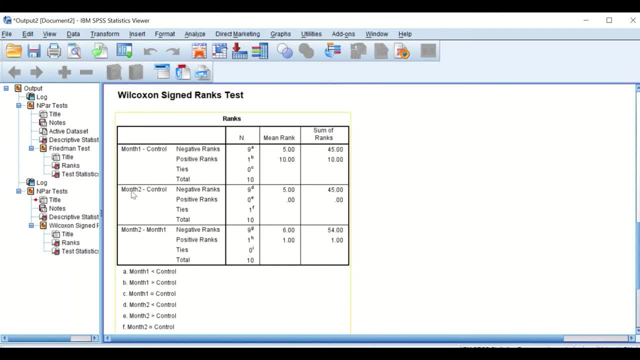 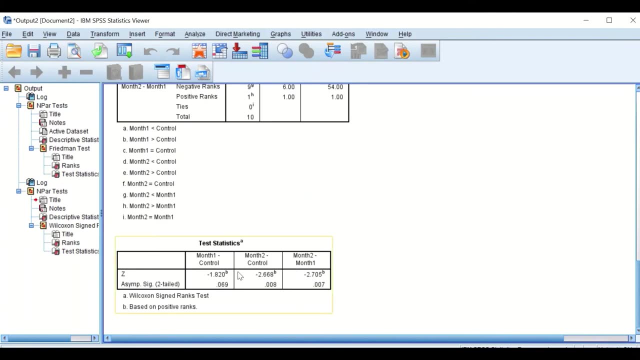 The data in one month to control and two months into control and one month to two months, And it works out the mean rank for each combination of group And we scroll down to the last Table. we see here that Wilcoxon has worked out the value for comparing two groups. 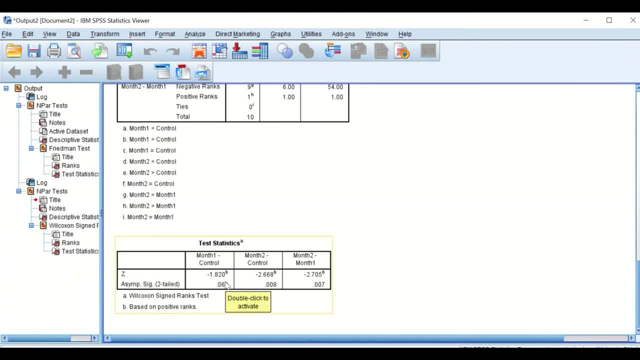 Month with control Here it does say there is no significant differences As there be valueless more than 0.05.. However, control with two months there is significant difference And with one month and two months there is a significant difference. 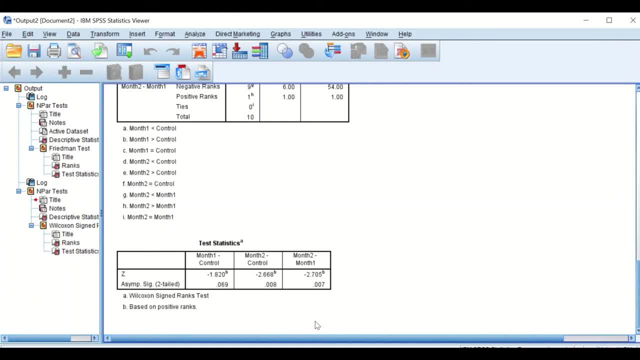 So this is really the way to find out which groups, Two groups, have really significant differences or do have significant differences when they compare to each other. So if you are using Friedman, you probably need of anyone to further detail and further information on if there is a significant difference. is to do, followed up by Wilcoxon signed rank test to follow up and find out which two groups really had a significant difference and which are not. 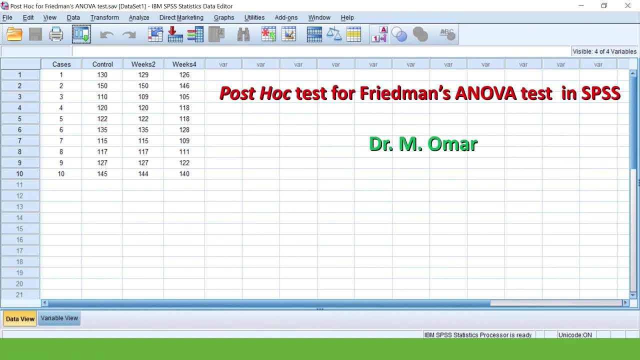 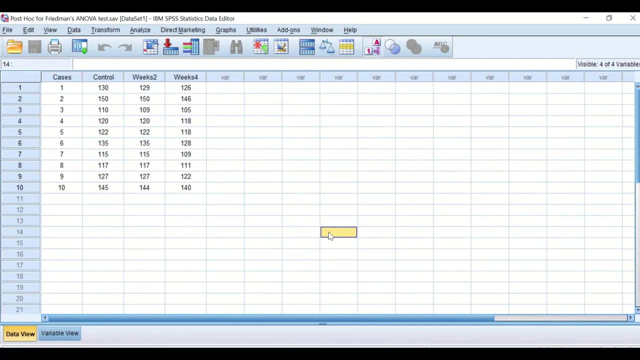 Finally, the post hoc test can be done Following a Friedman ANOVA test as a complimentary test. Here I have. I have a data from a company that has introduced a drug Wanted to test the effect of the drug on an individuals. You are in a period of time from two weeks to four weeks. 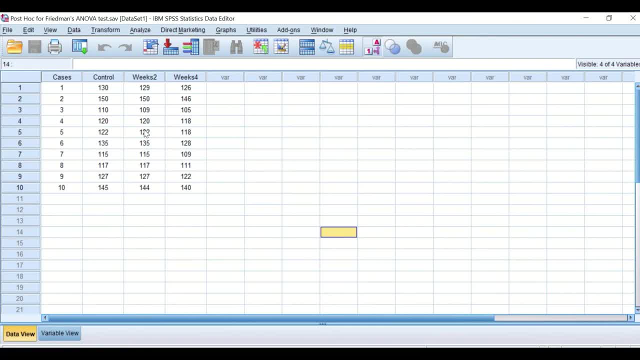 And to follow that by looking at the body weight, The body weight of an individual. So a drug designed to supposedly reduce the body weight. So in this study we have ten cases, ten participants, and every one of them Participated in all the measurements at the zero point or at the beginning of the test or a trial of this drug. 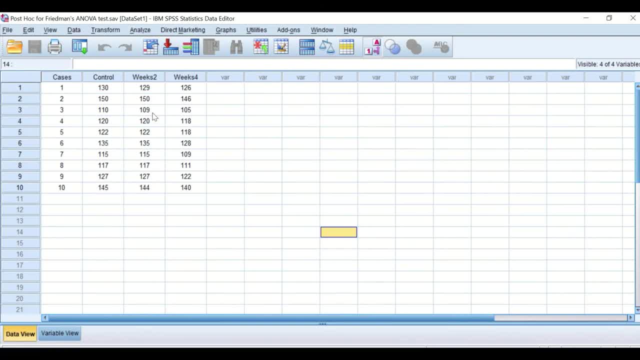 The weight for all the individual has been measured and taken. After taking the drug for two weeks, Their body weight was were remeasured again And after four weeks, the body weight was weights for all of them were determined. These data, as we can see, the sample size is too small. 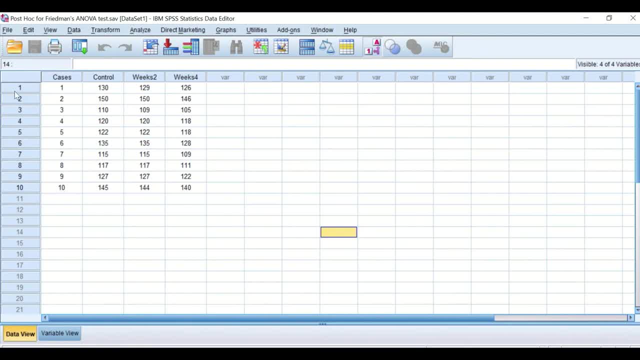 Ten samples And these, each individual, participated in all the other measurements. So they are related, The variable here are related And these data, These data in each group, is not normally distributed. So thus, if we want to find if there is a significant difference between taking a drug for two weeks or four weeks on the body weight, 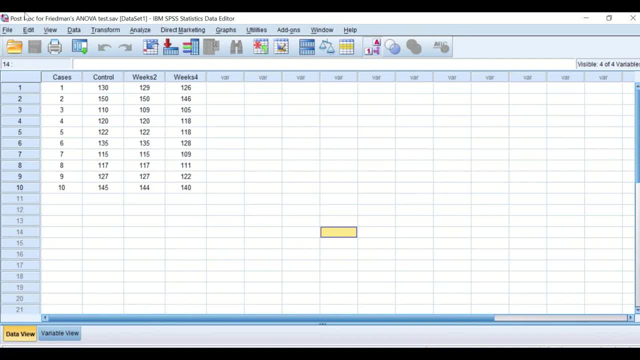 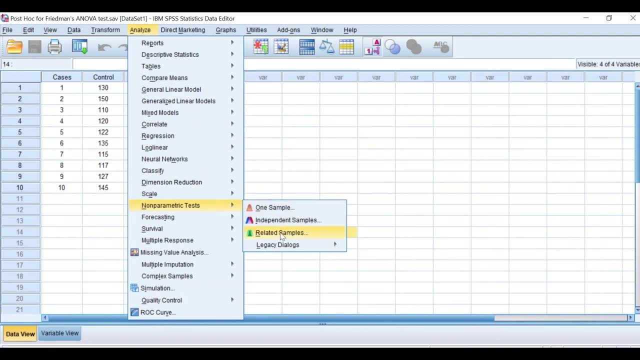 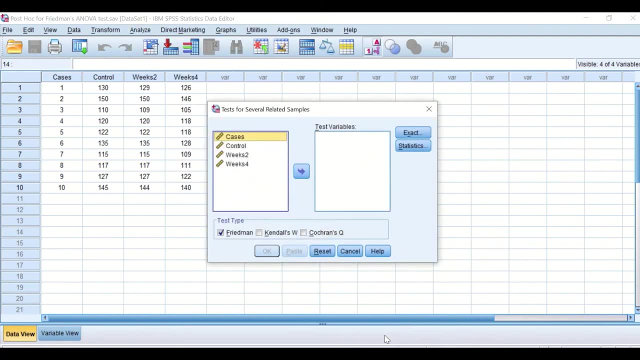 The best way to do it is to do Friedman ANOVA test, And to do that we click on analyze, Scroll down to nonparametric test And again to legacy dialog And then scroll to the K related samples. Here another windows appear. 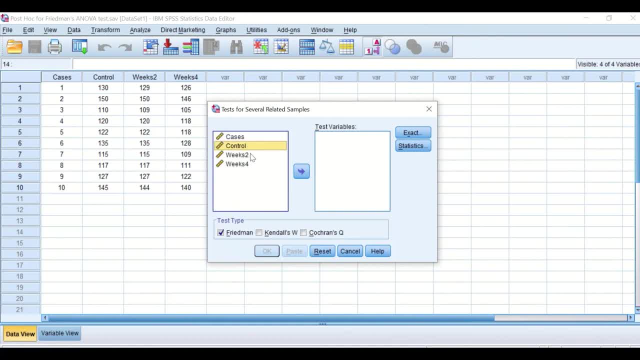 We need to select the control weeks two and weeks four And transfer them into the test variable To test for several related samples And, as we can see, we keep this Friedman ANOVA icon clicked on. If we click on exact, a window will pop up. 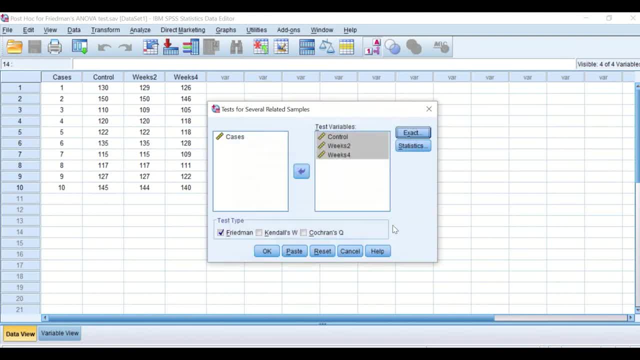 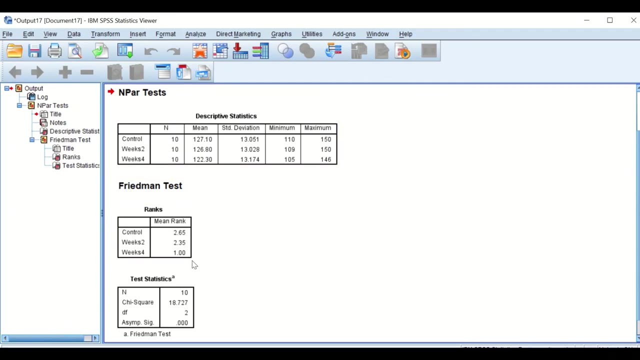 We will just leave it as it is And click on continue. Statistics will pick up and click on descriptive And then I will click on continue And then hit the button for OK. SPSS generates an output showing you that there are ten cases. 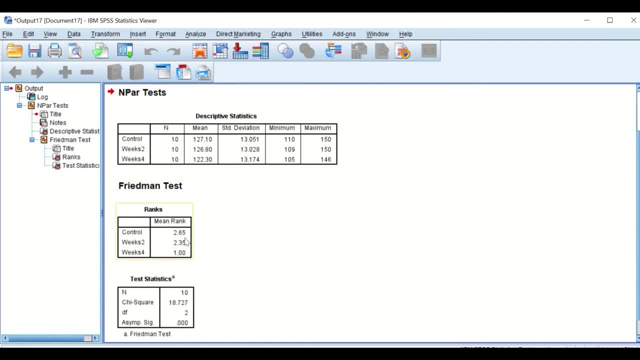 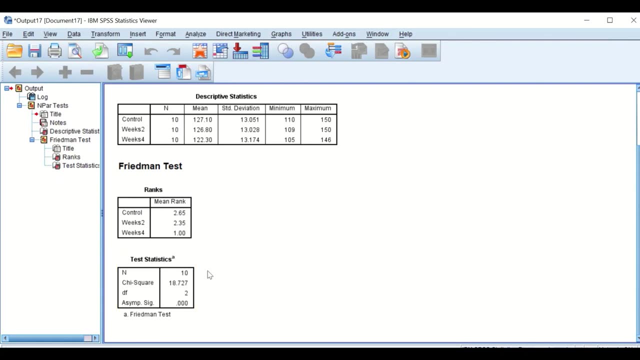 And three groups, And SPSS Friedman ANOVA took the data for each group- Actual data- And rank them And then give the mean rank for each group. Again, these data show that there is a significant differences between all the three groups. 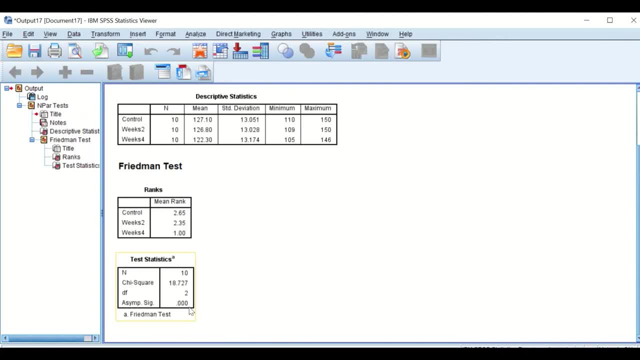 But again, it's an overall significant but doesn't specify what is- if there is significant between control and weeks two or control and weeks four. And the way to do that is, as I said in a previous video: You can do it through Wilcoxon signed rank test or post hoc. 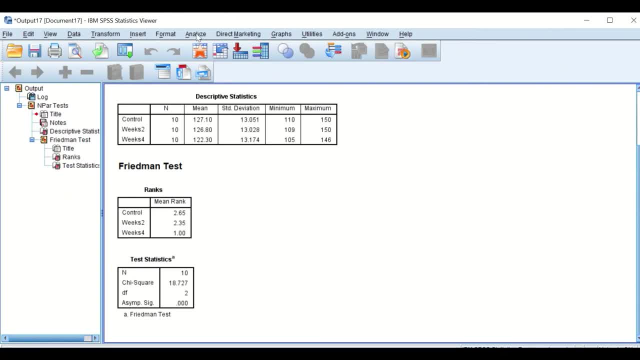 Here I will show you how to do post hoc test. So again, we click on analyze, We scroll down to nonparametric And then scroll down again to click on that test which is called related samples. If you double click on that, a window will come up. 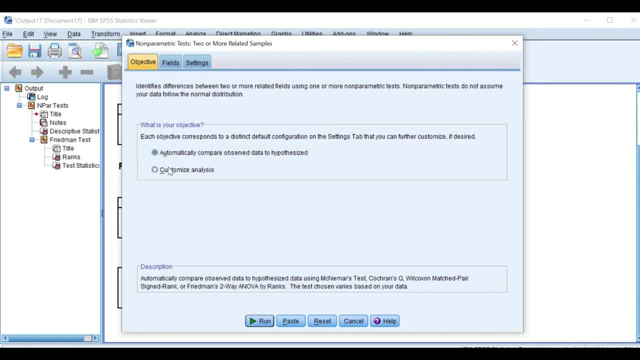 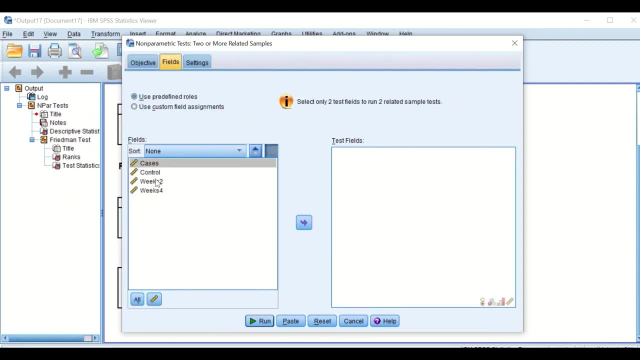 It's asking you What is your objective. I say click on. I just want to customize the analysis. Then go and click choose the field. Again, these are the three fields that I want to choose and I want to test, So I will transfer them to the right box. 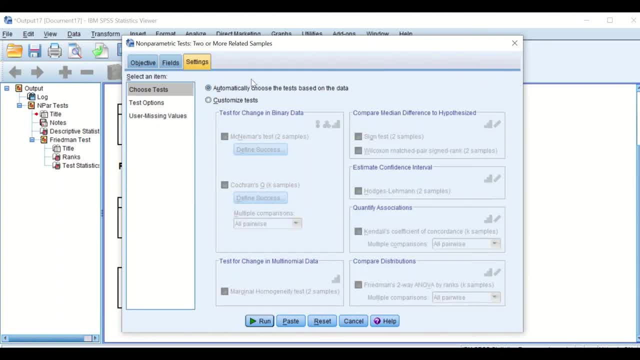 And then I will also click on the setting And in this setting, in this window, I will also select customize test. I will scroll down here and click on Friedman and over by ranks. Okay, samples, and all giving you all by pairwise. 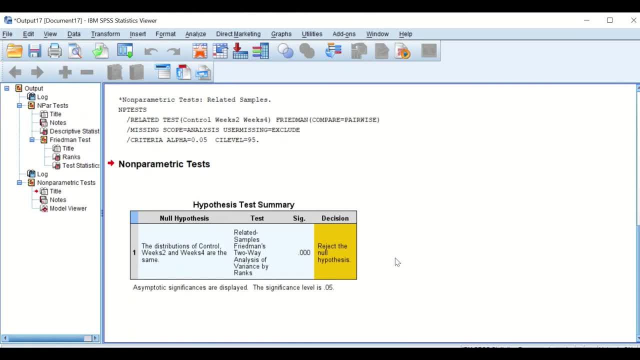 Then click on run, A box will appear showing that there is a significant difference between the three samples And it's really put in hypothesis And it says that there are significantly less than 0.05.. If you double click on this table, 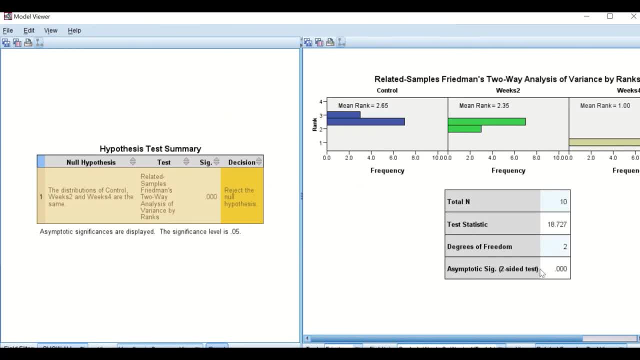 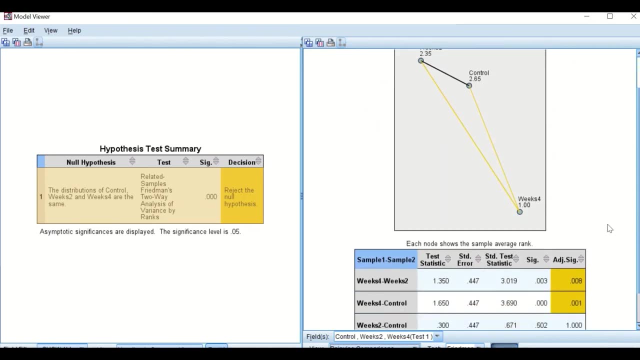 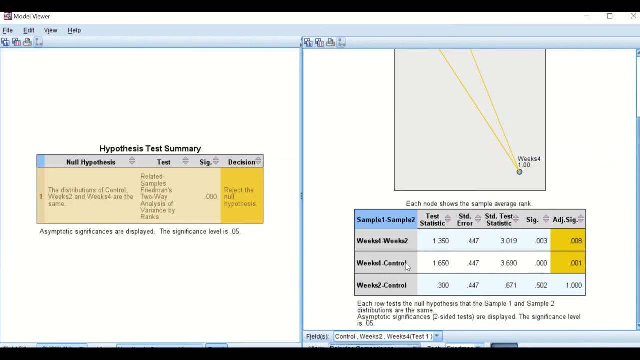 Get another window here next to it, showing the control, the week two and week three. If we scroll down to here and click on pairwise comparison, another table will appear And this table really is showing the comparison between control and week two, control and week four, week two and week four. 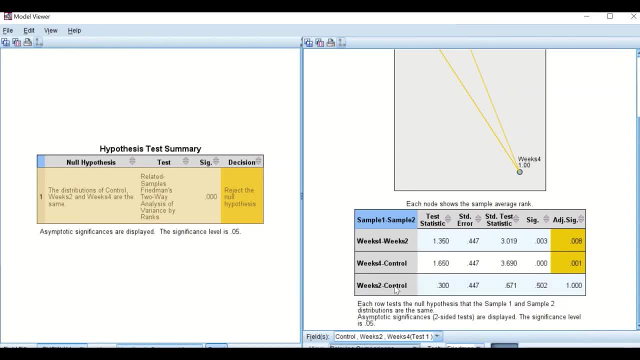 Again These, as we can see here with this post hoc test, It shows that there is no significant difference between control and week two. However, because the P value is equal to one, However, there is a significant difference between control and week four. 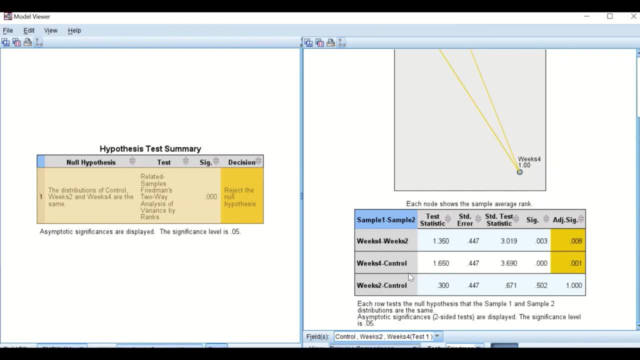 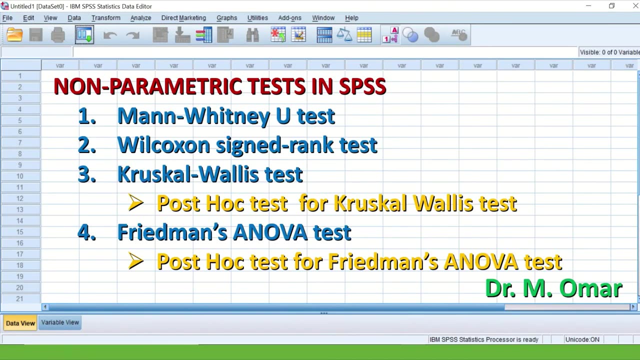 So and those saw some significant difference between, also significant difference between control and week four, As the P value is less than 0.05.. So, as a final recap, there are four major nonparametric test in SPSS, Which one to use depends on the group you have with that. you have two groups or three or more groups. 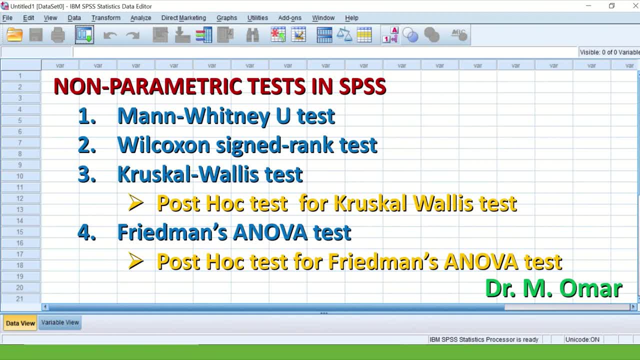 And whether these groups are related or not. If you have two groups that are not related, then Mann Whitney U test is the one to use. If the two groups are paired or related, then Wilcoxon signed rank test is the one to choose.